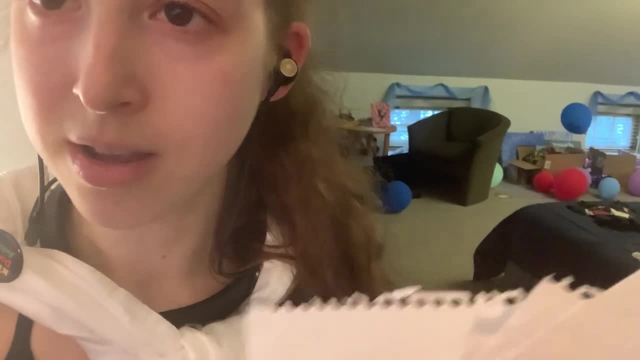 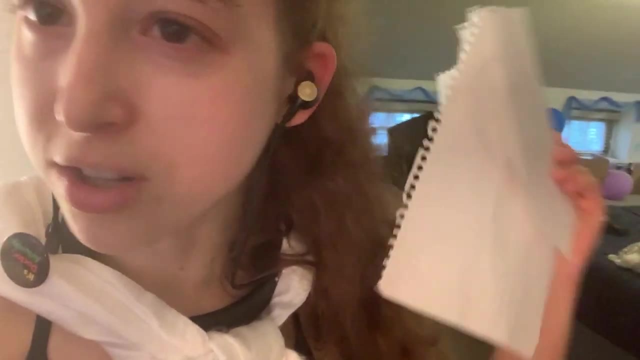 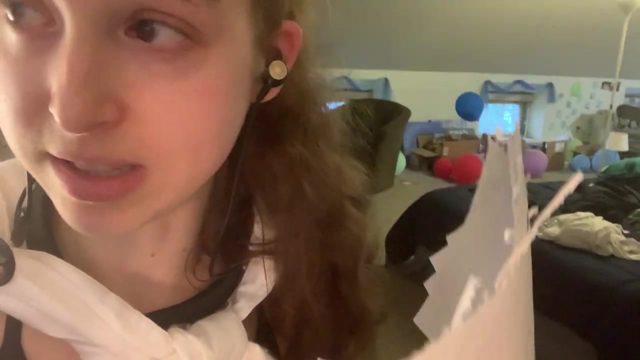 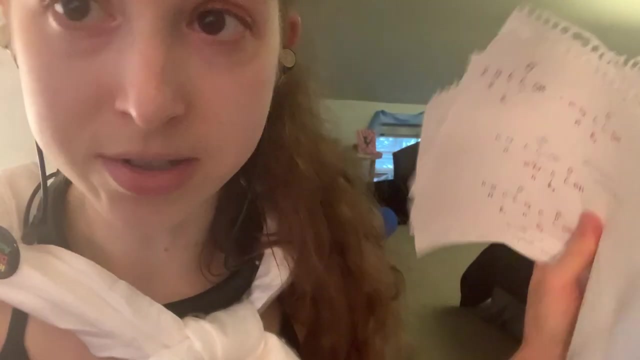 activate an amino acid to make it more reactive. So you add it, react it with ATP, you add the AMP part on there And then you're going to, just from then on, you're transferring that to other places. So you're going to transfer it to TNA, TRNA, which is going to give you the specificity. you need to make sure you're adding the right letters, the right amino acids that correspond to the mRNA, And then you're going to, with the help of the ribosome, catalyze the transfer. 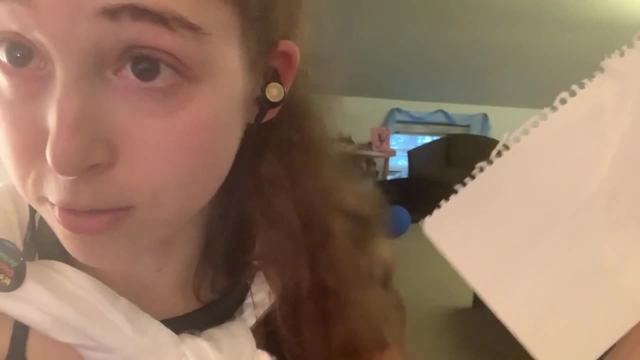 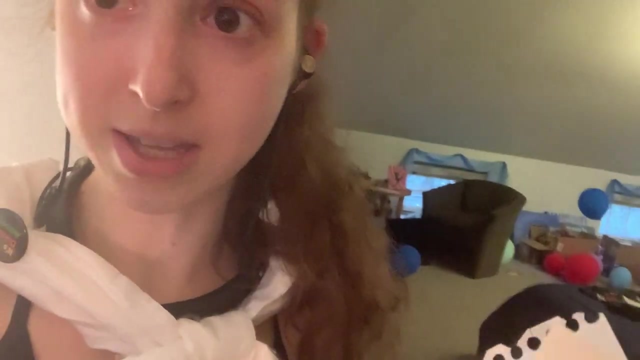 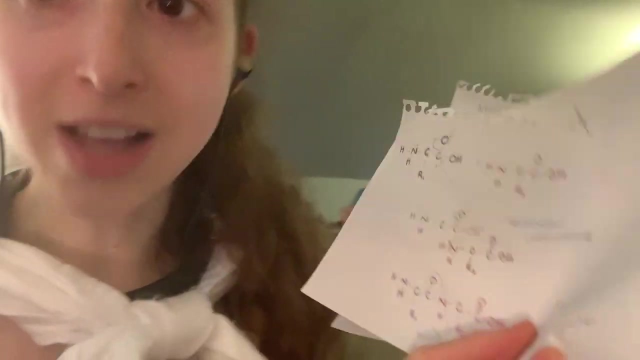 of a chain that's of peptide previously formed, peptide bonds like so a peptide that's already forming. you're going to transfer that onto the incoming tRNA, which is charged with the amino acid, And so you do end up losing the equivalent of a water molecule, but you're not actually losing. 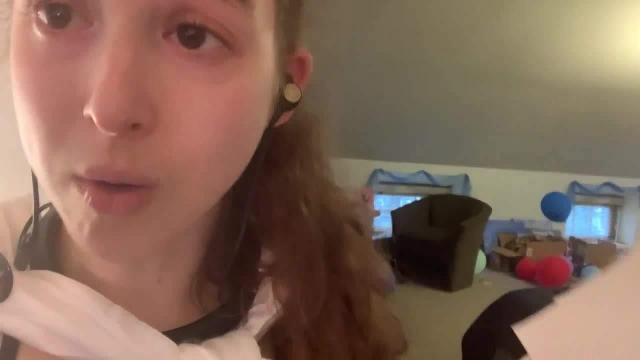 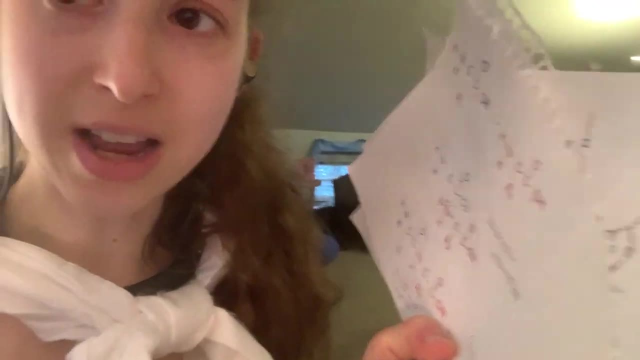 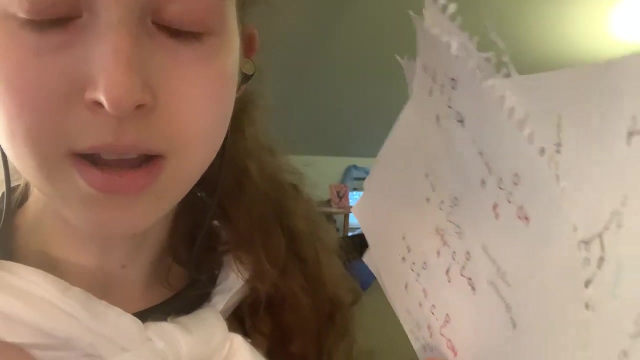 it as a water molecule and you're actually losing parts of it along the way, And the reaction is pretty cool And I wanted to kind of just walk people through it. So this is going to be another one of those really technical ones And with like arrow pushing and stuff, And so I'm not 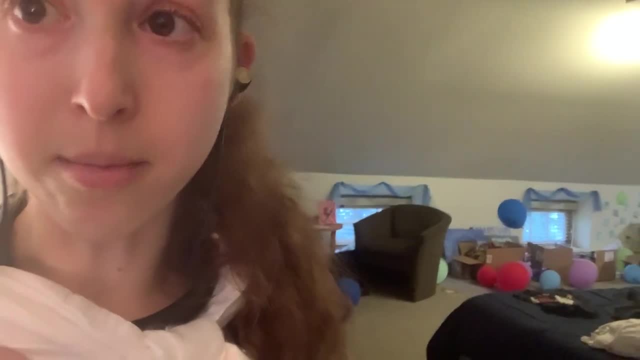 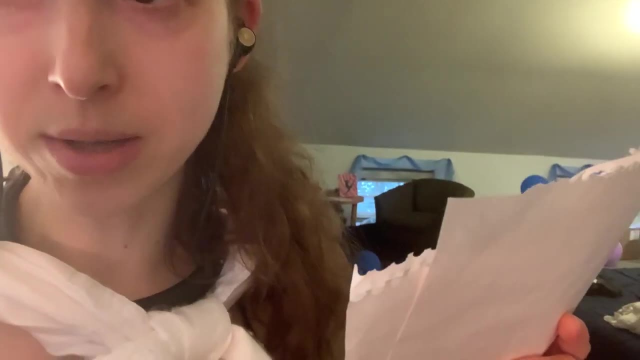 going to explain things as much as I normally do. Sorry, But hopefully this post will help people like me who always got confused when they're like: but this isn't how it really happened. Okay, so in chemistry you might see something like this. So you have this. 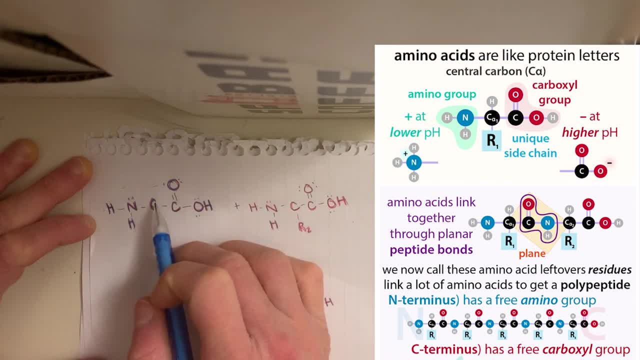 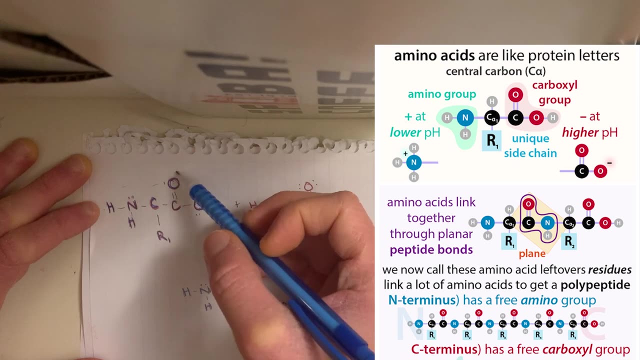 amino acids, And so we're going to. this is: they have that. this is the generic backbone, and then their unique side groups, which I'm just going to abbreviate R1 and R2.. And I've tried to color code things so you can see where things go. So this is our first one, And so you can see we have this. 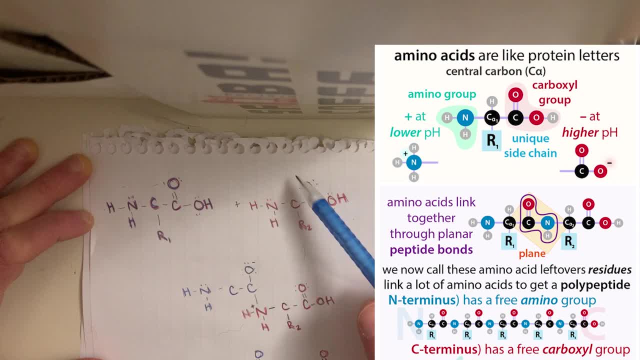 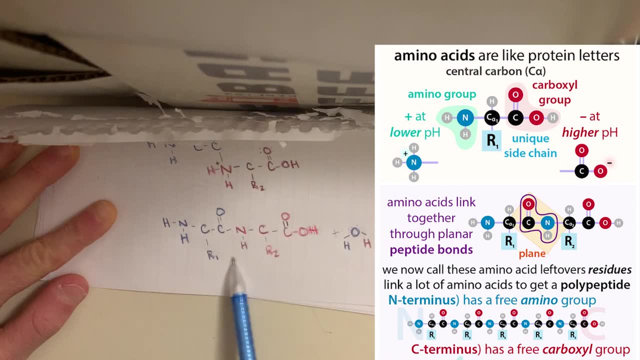 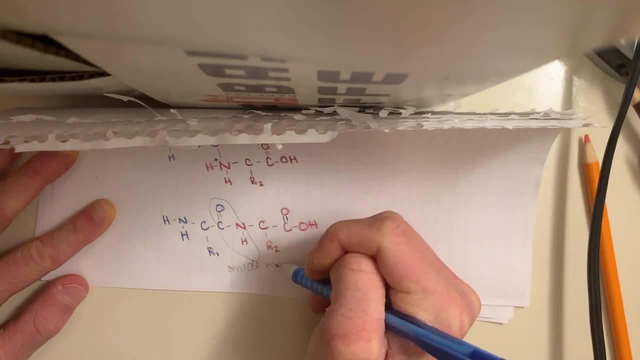 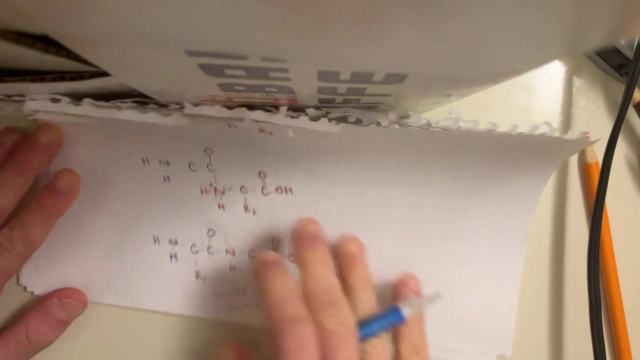 carboxylic acid group and this amino group, carboxylic acid amino group, And what we're going to end up with is this: This is our amide bond, Which is we call it a peptide bond in this case, But it's an amide bond. 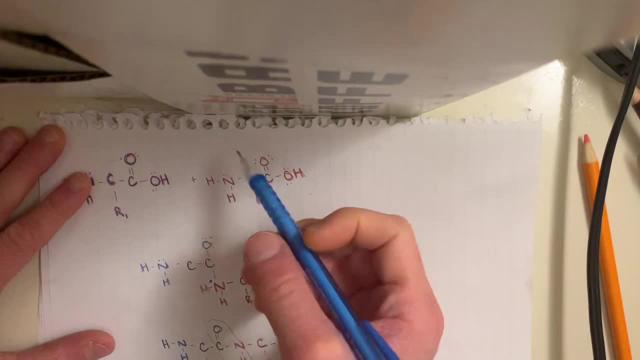 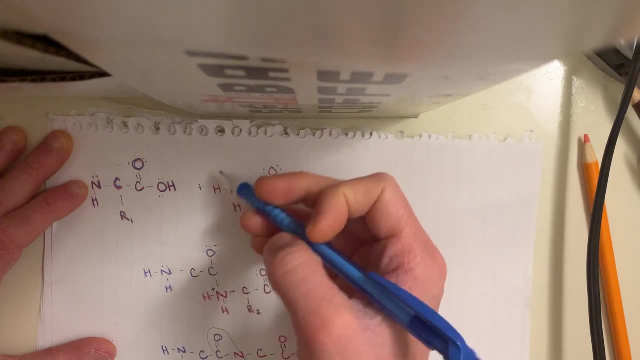 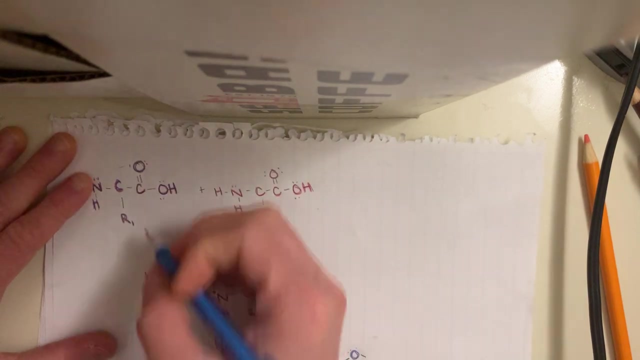 And we're going to call this reaction. Let's see what, how this reaction could go and what we're losing. So if you look at this here, you could have imagined. So remember that the oxygen is electronegative, So it's pulling electron density away from this carbon. So this is going to be. 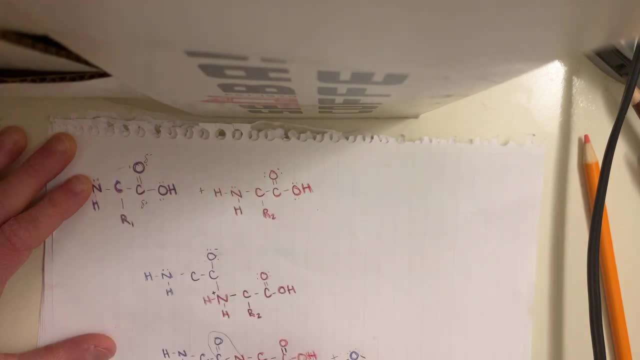 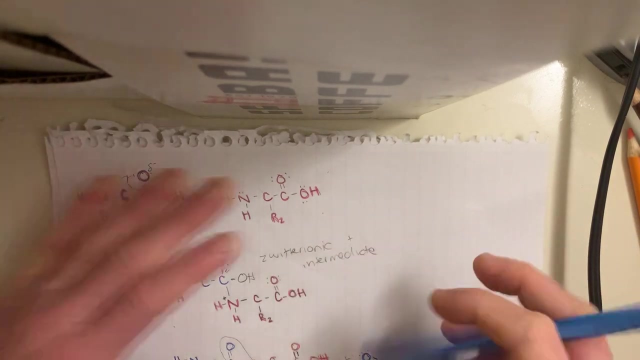 partly negative And this is going to be partly positive. you have this lone pair of electrons on this nitrogen. this can act as a neutral nucleophile. The electrons are going to flow up to the oxygen. get your single bond and now your have this weird. 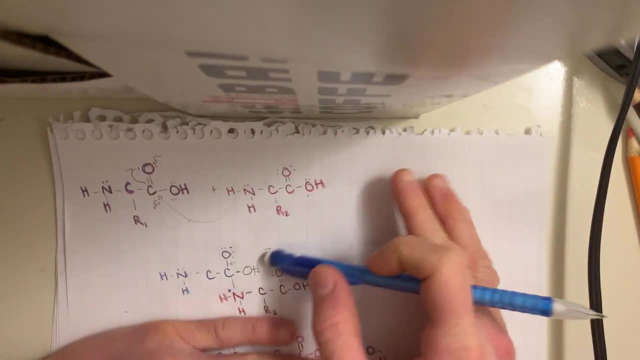 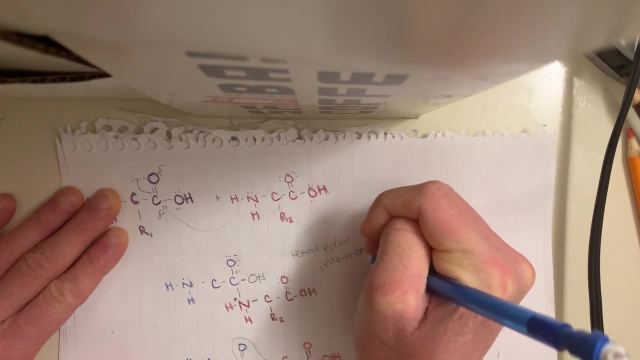 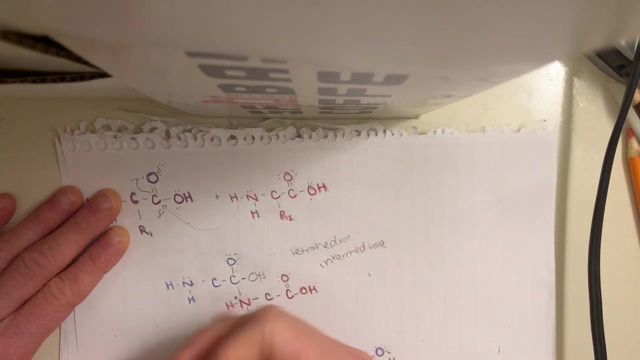 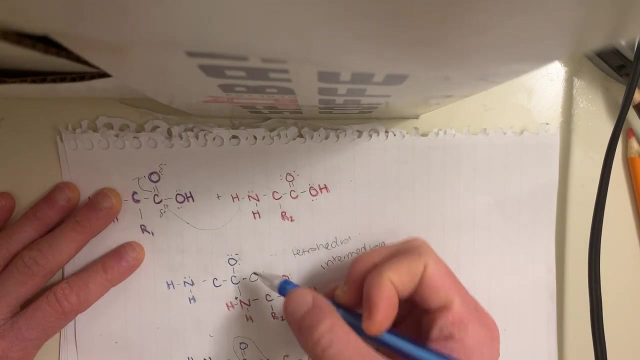 weird tetrahedral intermediate And this is going to be an unstable intermediate. You can see it's kind of crowded and you have this separation of charges and it's not very happy. So what you can get is you can actually have the oxygen. the lone pair is going to flow back to reform that double. 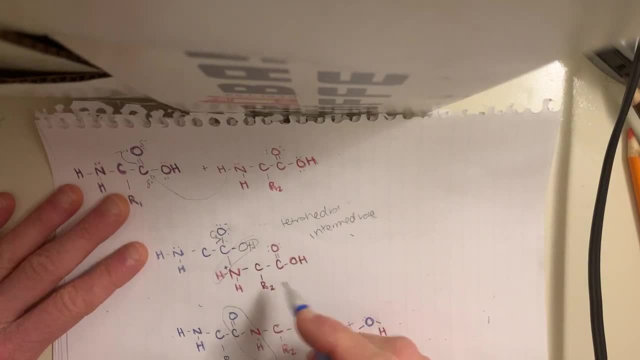 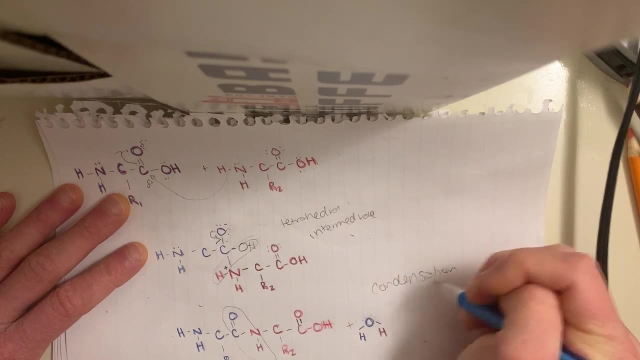 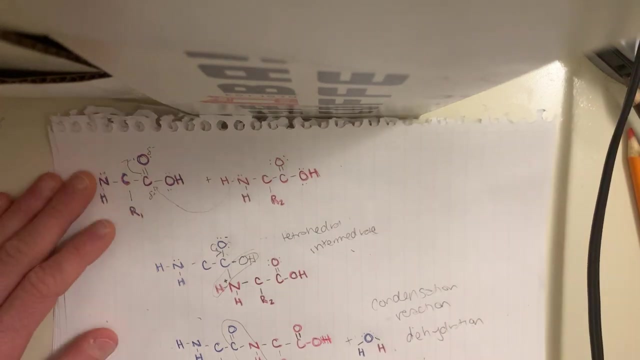 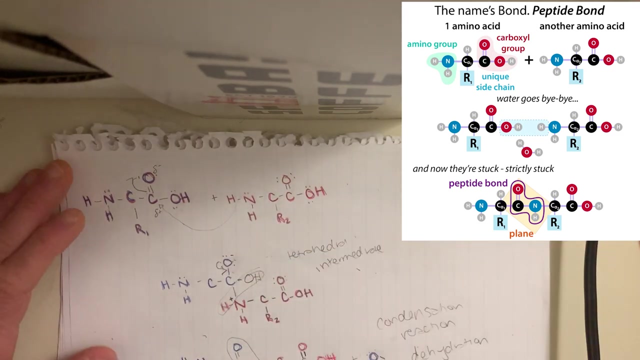 bond And this OH is going to leave with the hydrogen as water. So this is a condensation reaction or dehydration. You're losing water. You see, you have the two. you have this OH from your first and the hydrogen from your second, and all is good right, Except things really aren't. 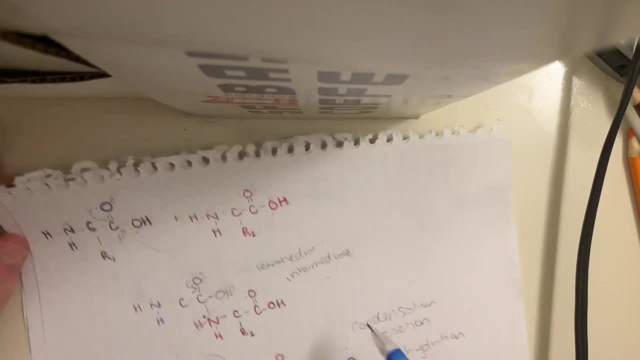 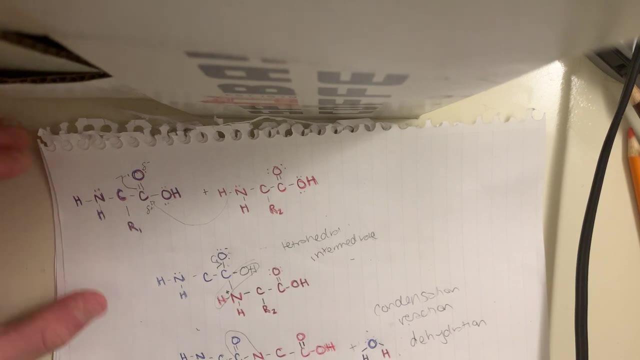 that simple And so when you learn this reaction, say like: well, this isn't actually how it actually happens in your body And it's not in our body. It's done on the ribosome and it's done with the help of the ribosome acting as an 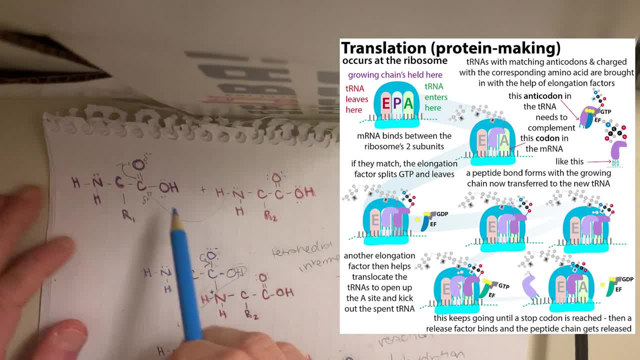 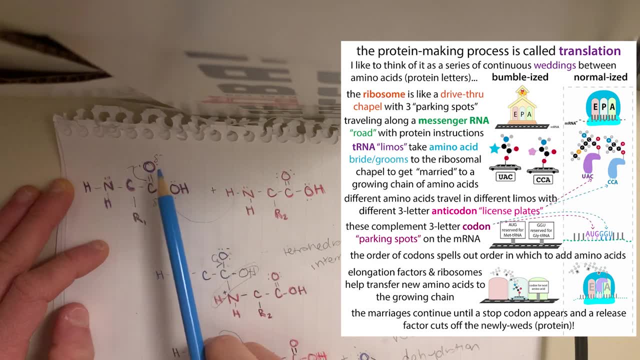 enzyme. So it's going to speed up the reaction And it actually happens first, though It happens through several intermediates. So you're actually going to use ATP to charge your to activate the amino acid. So basically, we need to do like a. 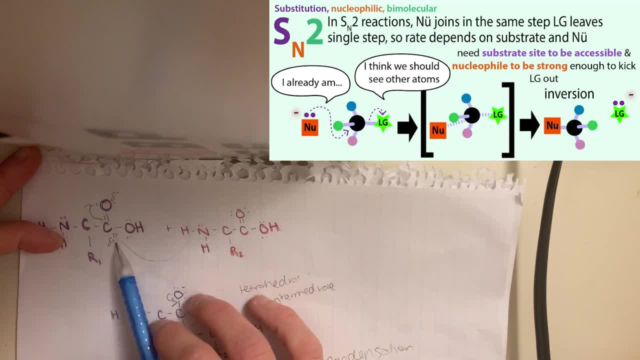 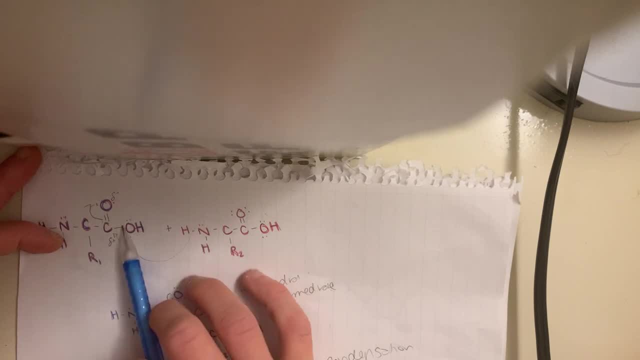 substitution reaction. We're going to substitute out this OH group for this part, but to do that requires this part to leave, So it's a leaving group and OH is a bad leaving group And so when we do it in our bodies, we make this a better. we can activate this by making a better leaving group. 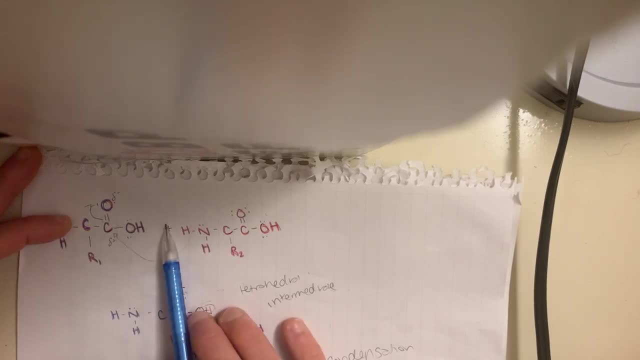 So we're going to switch this out for, um, AMP, and then that's going to be a much better leaving group because, although like so if we have this, we can get this oxygen to react to things, um and like, add on to things it's harder to get. 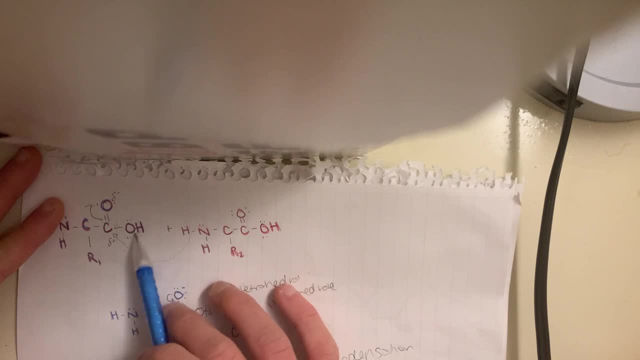 this group to leave Um. so- and we don't want to- if we get that oxygen to react to things, we're going to make a bond to the oxygen and we end up um with an ester, but we don't want an. 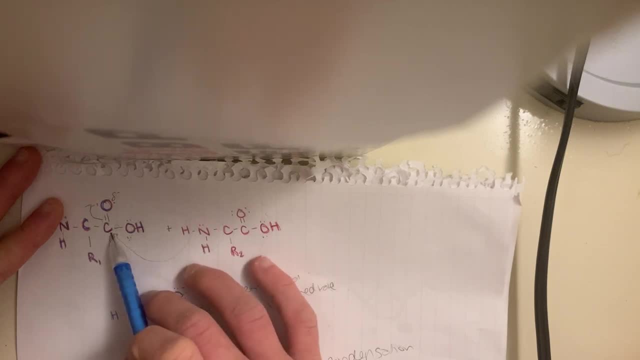 ester. We want an amide, We want this, we want to react directly to this carbon, And so to do that, we're going to need to activate this group and make this um a better leaving group, So it can go bye-bye when you make the. 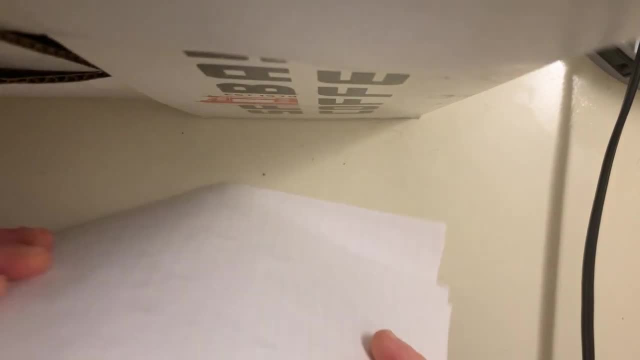 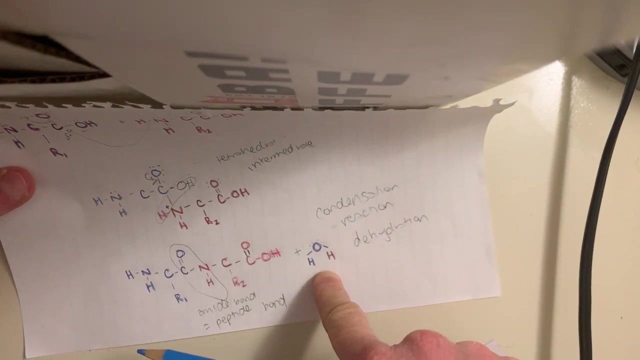 new bond here. So how we're going to do this is we're actually going to use ATP to get energy and we'll still end up with that same final product. So we still will get a um. we still will get the loss of equivalent of a water molecule. 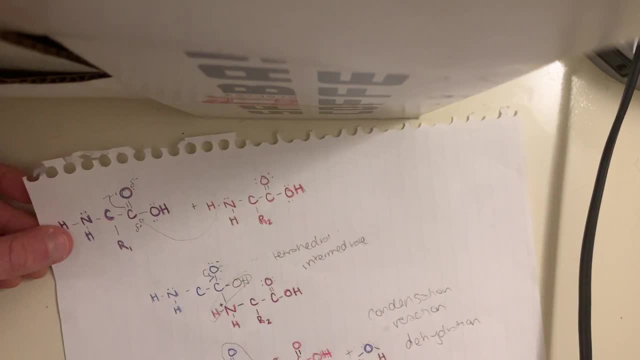 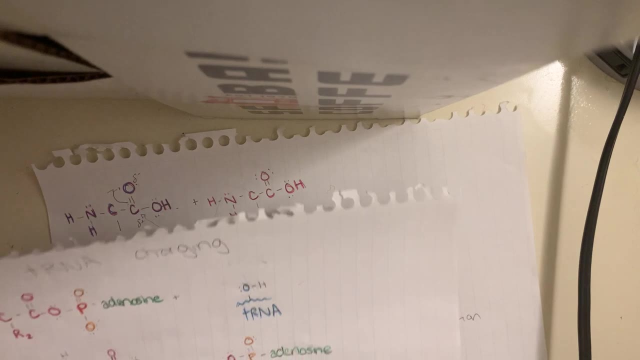 but we're not going to lose it like this in this way. Um, we're actually going to lose it kind of stepwise and we're going to. the water is actually the oxygen is actually going to be lost during the tRNA charging step, Um. so in addition to activating it with the um, so basically our 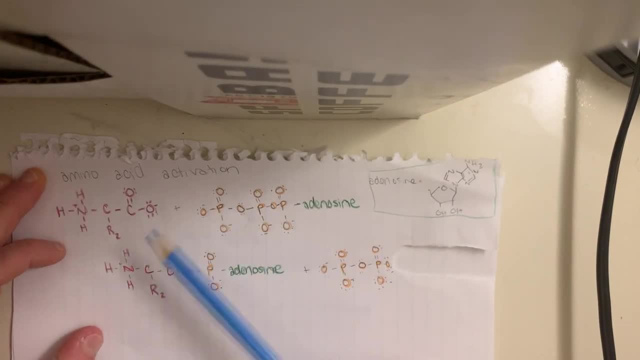 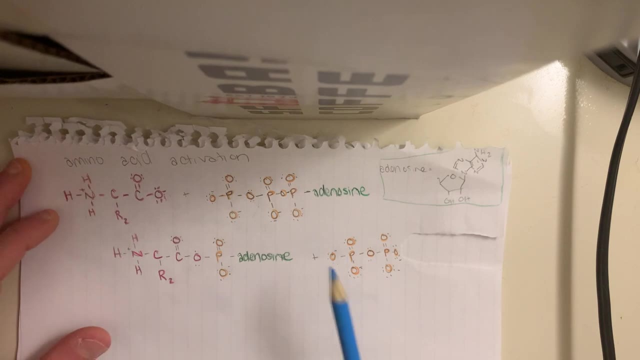 first step is going to be to activate the amino acid. So we're going to swap out this um carboxylic gas group, We're going to attach it to an AMP, um from ATP, and then we're going to. 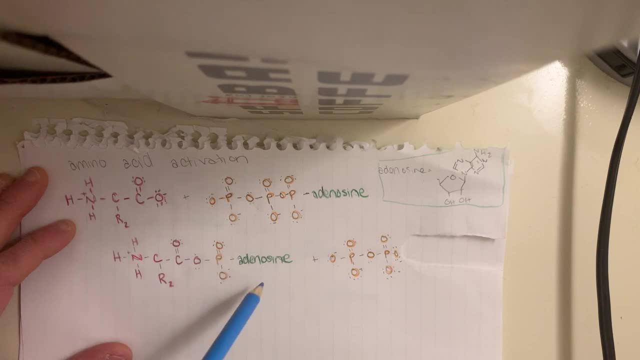 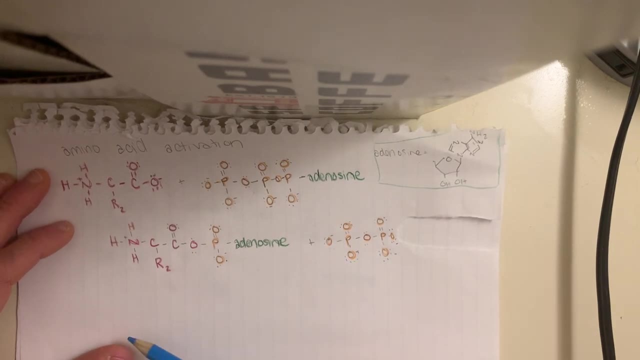 the rest of this group is going to be activated. So we're going to attach it to an AMP from ATP and it's just going to be transferring it to um other, transferring it to other things. So we're going to transfer it to tRNA. then we're going to transfer it from that tRNA to another tRNA. 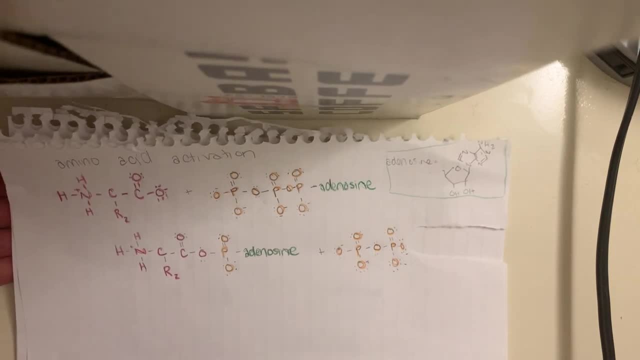 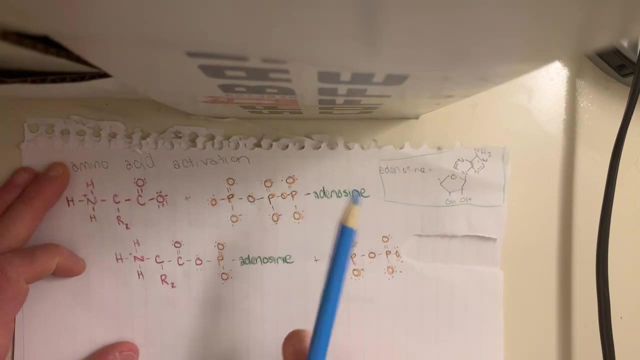 That's what the growing chain we're going to go um, or that's the incoming tRNA, Um. so you'll see, it'll make more sense in a minute, hopefully, But yeah, so I've tried to draw this out, Um. 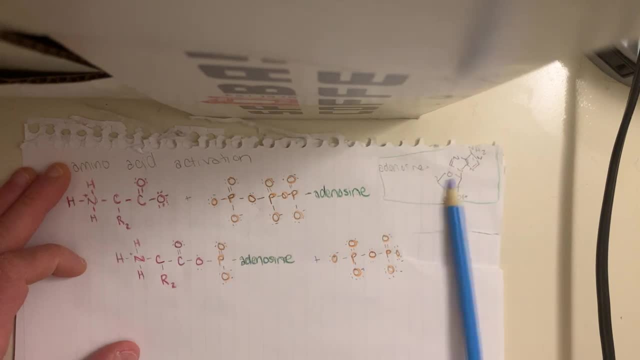 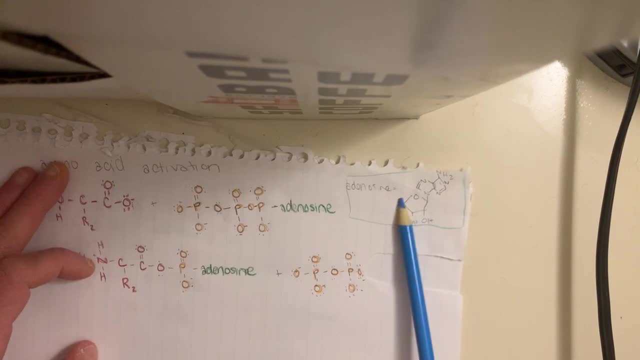 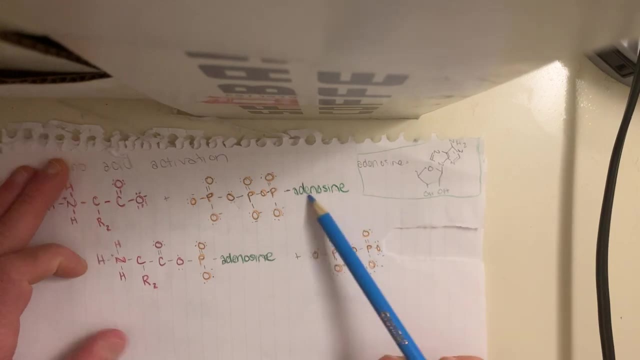 it's this um, this group. So you have this ribosugar and then this adenine, um, nucleotide base, Um and the. you have these three phosphate groups in a row um which are there. So this is. 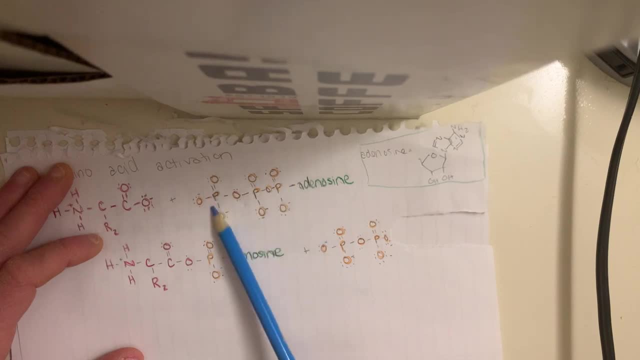 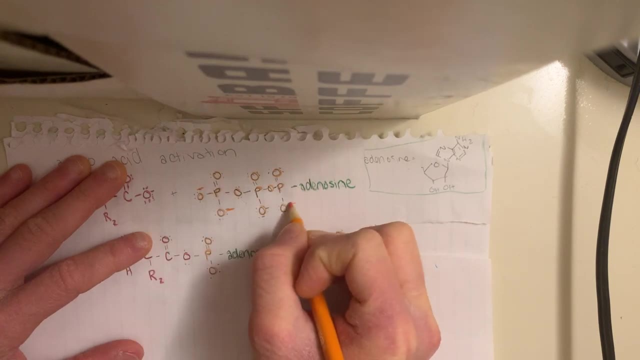 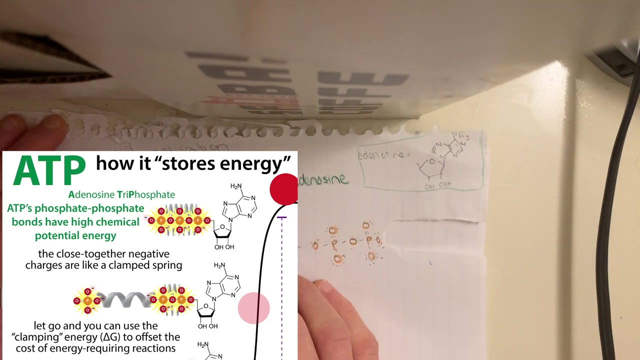 very high energy. This is very unstable. These are all negatively charged. It's kind of hard to see, um, but these are all negatively charged And when you have a bunch of negatively charged things next to each other, they're going to try to repel. So you have high energy in this. So, if you can, 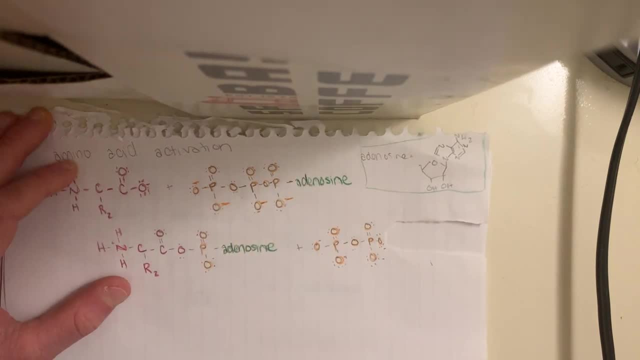 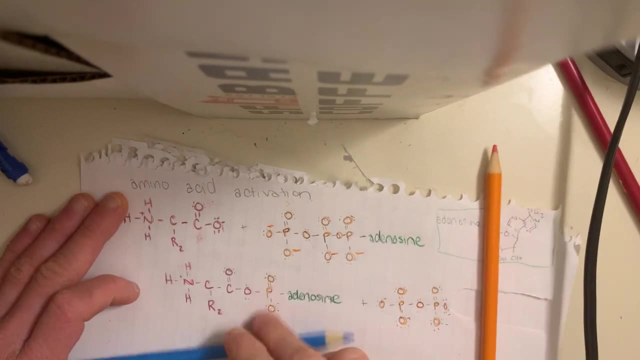 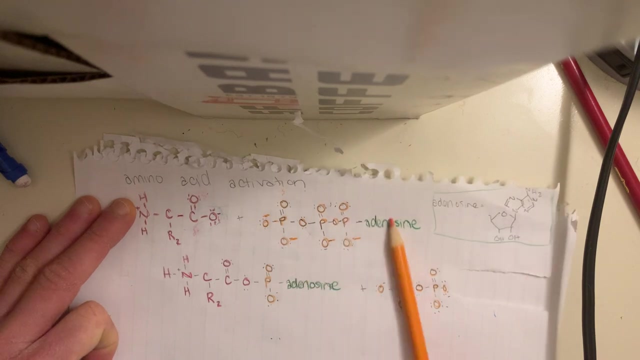 break these bonds, you're going to generate a lot of energy that you can use to do things like to form the um bond between the amino acids. Okay, So how are we going to swap out that um, this group, for the um, AMP? So adenosine, this is adenosine triphosphate, And what we're going to. 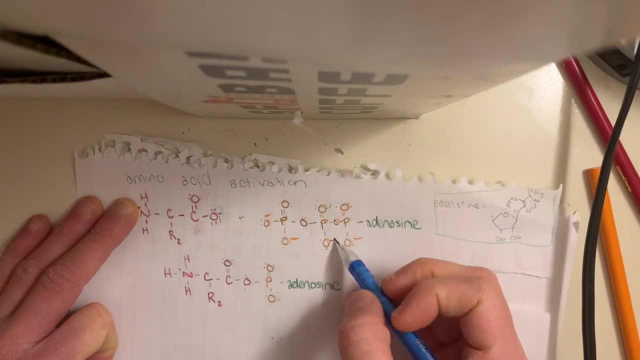 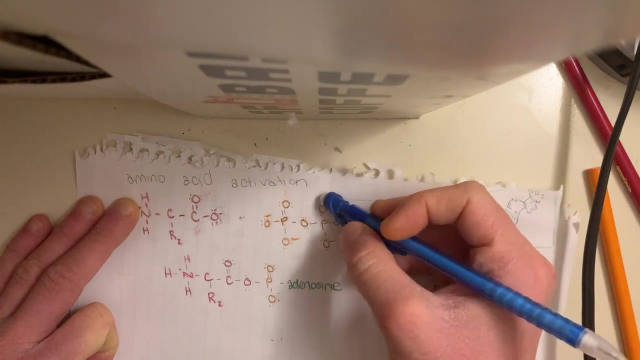 do is we're going to attach adenosine monophosphate, So we're going to add just the this part, um, but we're not even going to add that oxygen. We're just going to add that part. and how we're going to do it? We can do this because- so remember these, the, these want to. 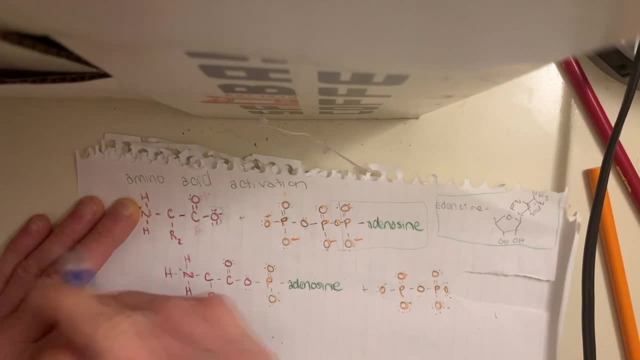 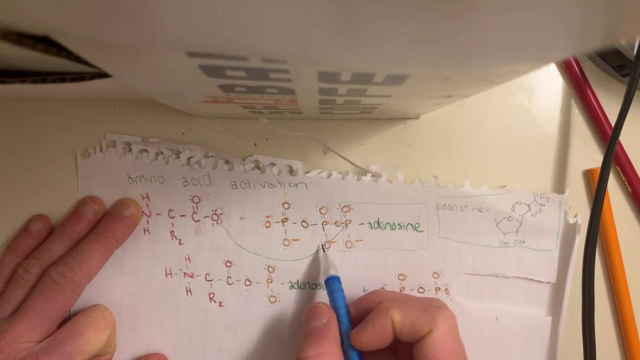 break. These bonds are going to be easy to break and that's going to give us energy, Um, these oxygen. here you have this negative charge, you have these lone pairs. It can act to attack this phosphate because so, even though this is really negative overall, it can act to attack this. 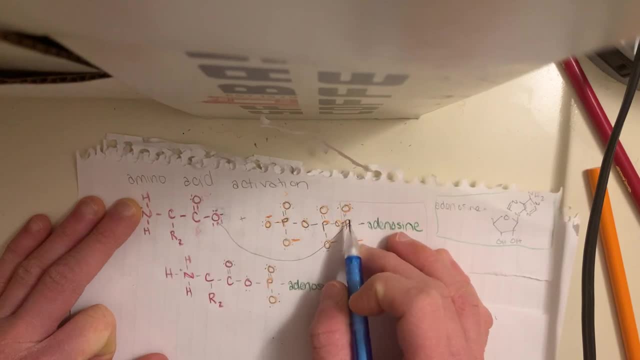 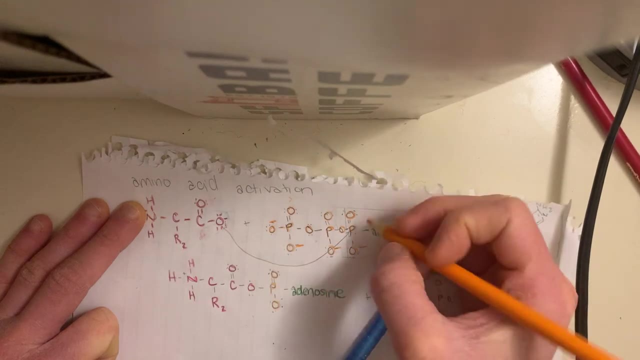 phosphate, because so, even though this is really negative overall, the oxygens are pulling electrons away from the phosphate, um from the phosphorus, And this is going to make um the phosphorus partially, um partly positive, And so you have this negative, you have this positive. 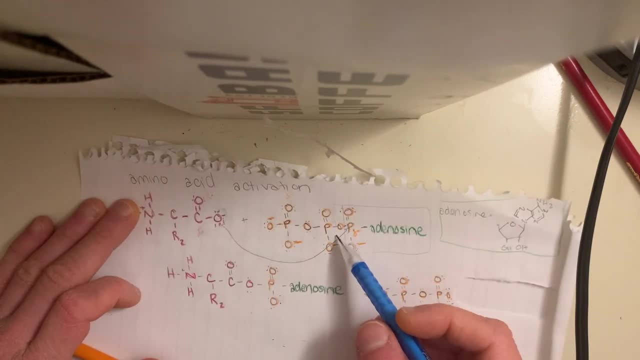 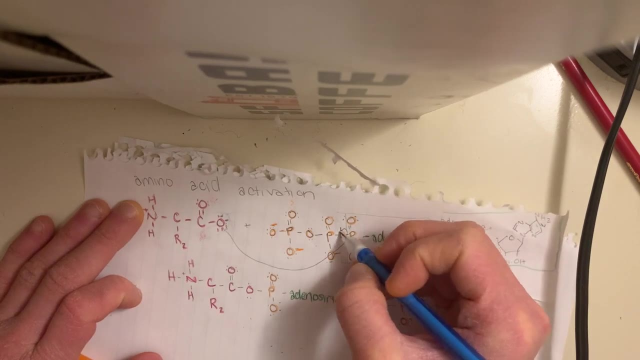 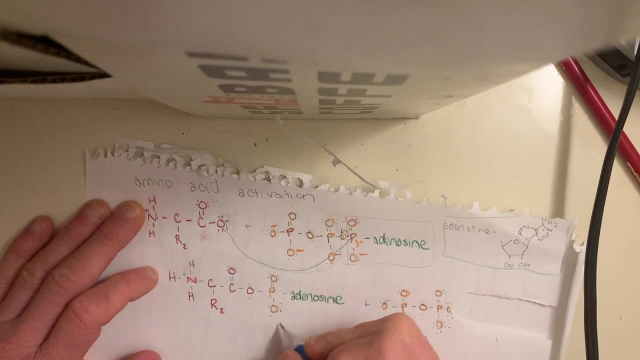 you have this lone pair so you can get this attack. When you get this attack, then this um is going to go here And this. you have this, leaving as these um PPI, and you have your AMP. So we started with ATP. 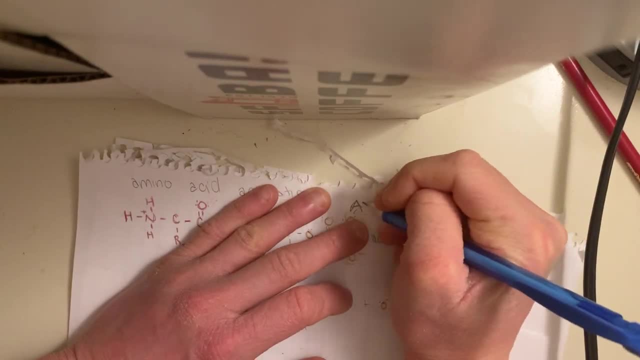 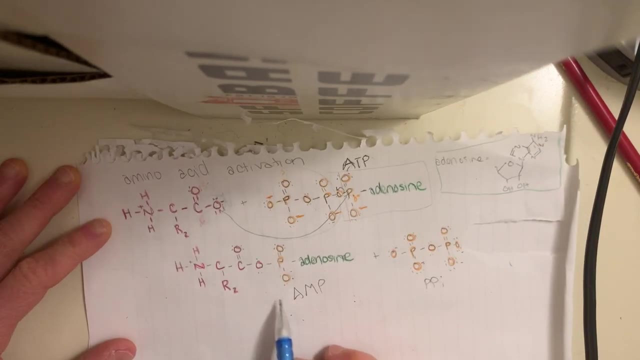 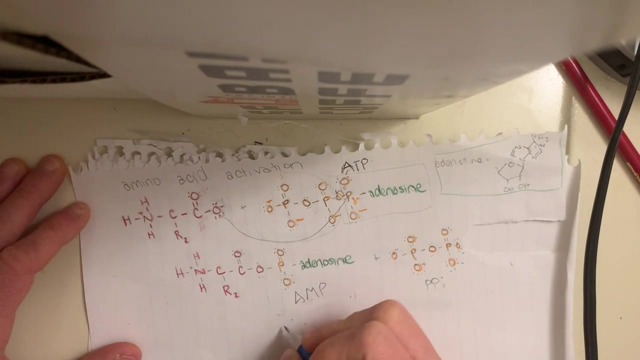 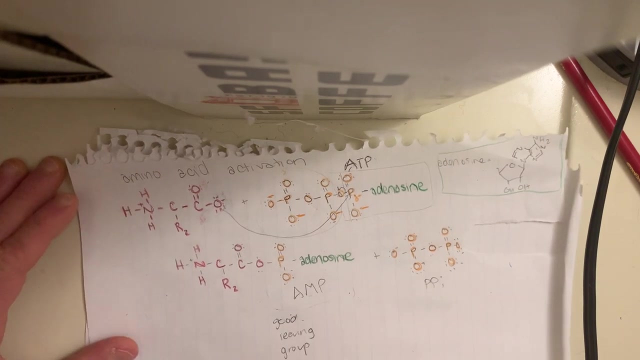 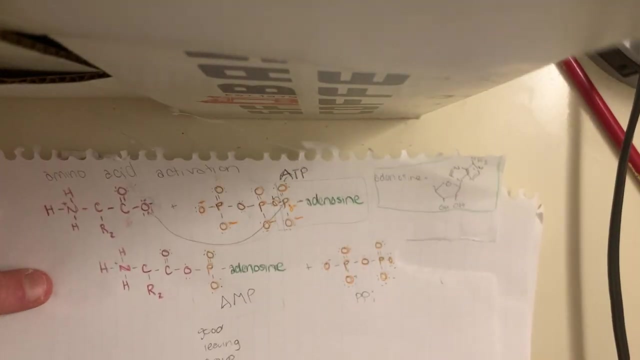 and we're only going to attach the AMP part. Okay, But now we have this better leaving group, So this is a much better leaving group than just an OH would be. So this is a good leaving group, So this is going to be reactive Um, okay, So now we have the. this step is called amino acid. 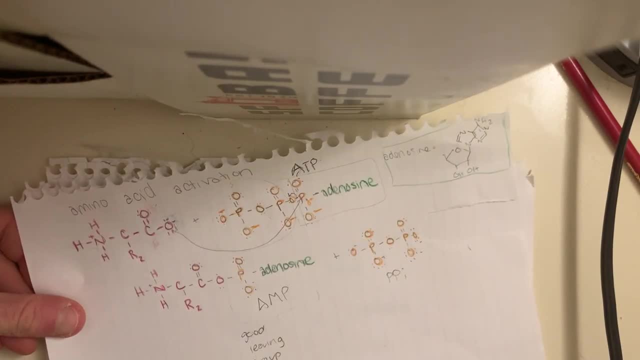 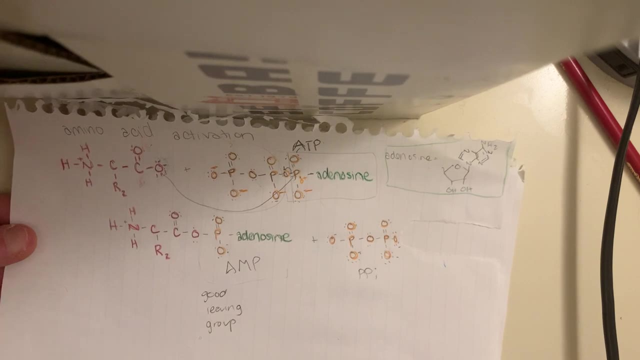 activation. We've activated this amino acid. We've given it the energy that it needs um for the reaction to happen, And so, for the rest of things, we're not actually going to add any more energy um to get this reaction to happen, but we are going to transfer it, and we're not. 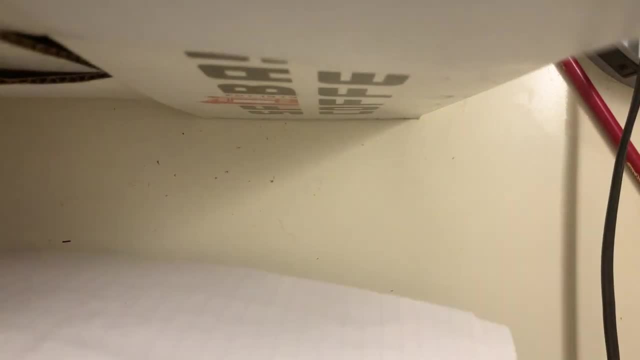 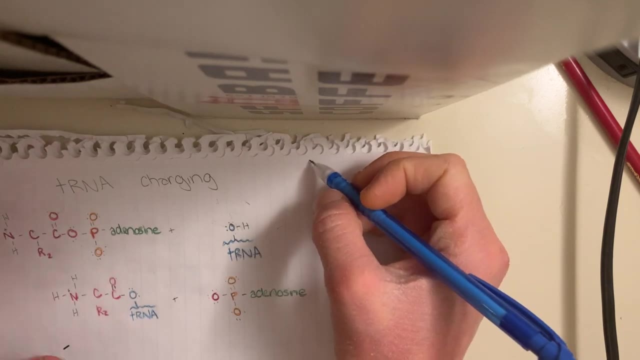 going to transfer it directly to the other amino acid. Instead we're going to first um, transfer it to a tRNA, And so the tRNAs. this is going to provide our specificity um and it's going to kind of give it a handle to be used in the um, in the ribosome. So remember, 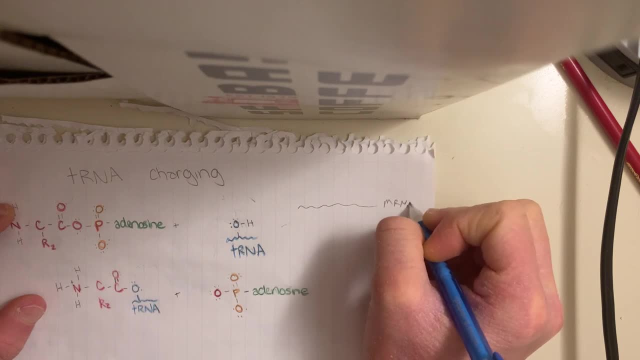 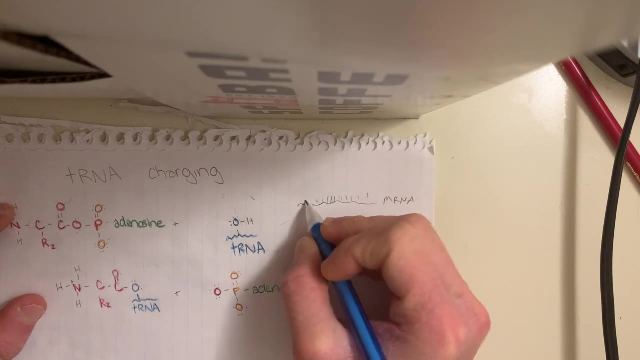 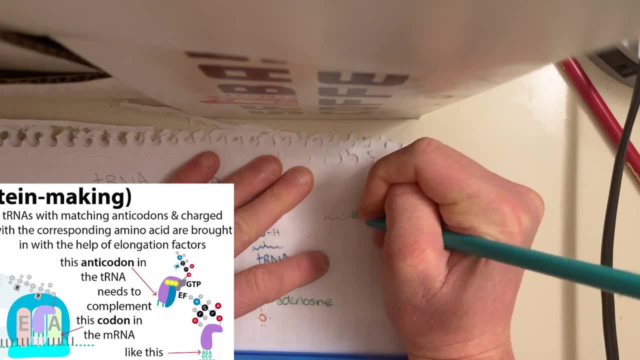 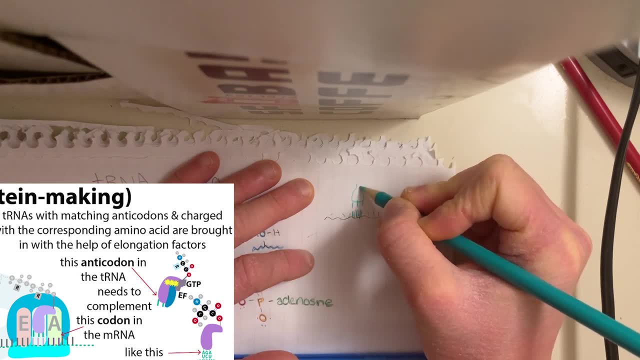 in three letter chunks called codons, And so you'll have one code on here and then your tRNA is going to have the matching anti-codon on it. So the tRNA, like the name sounds, it really is an RNA, And so it's going to have this anti-codon and then it's going to be attached to. 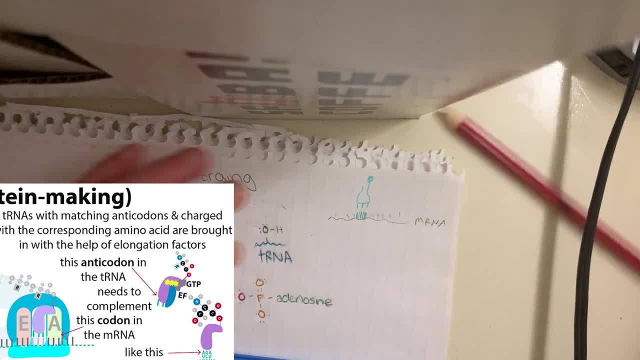 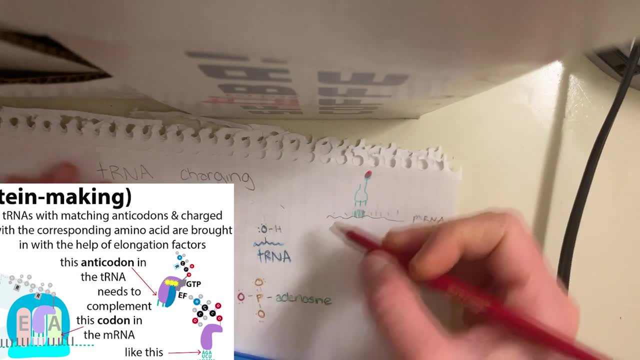 the incoming peptide, Um, and so I guess this would be red in our case, Um. so this is our incoming peptide and it's on this tRNA And so this is going to allow the specificity. So the amino acid activation part was activated in the amino acid, The tRNA charging part. 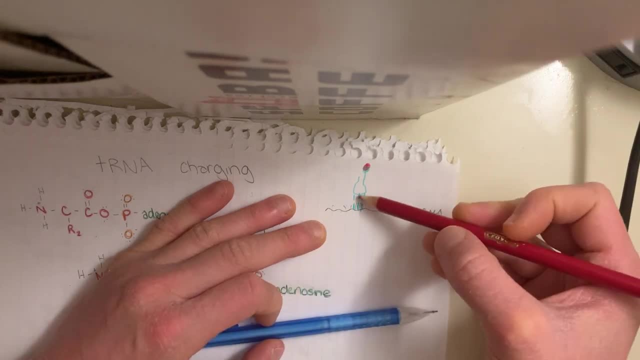 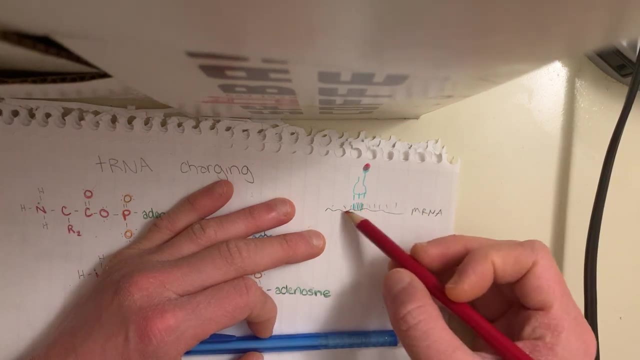 we're actually sticking the amino acid onto the tRNA And this is going to provide the specificity we need to um to make sure that we're giving the sequence specificity. So the mRNA is specifying the sequence, The tRNA has the matching anti-codon with the corresponding 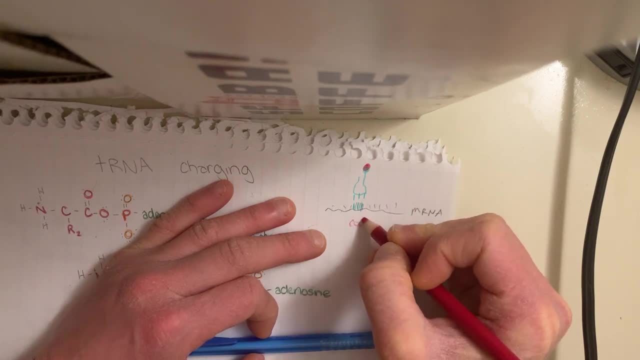 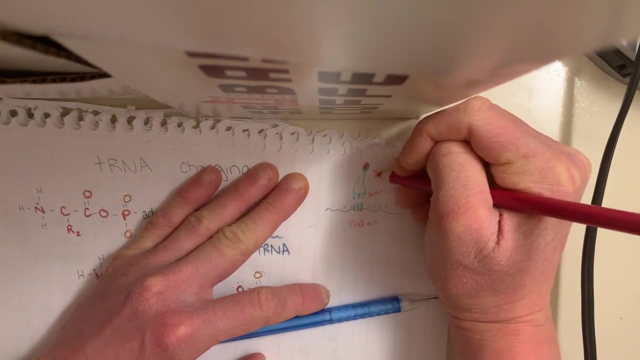 protein letter, So three. so this is the codon is in the mRNA, The anti-codon is part of the tRNA, And then this is the amino acid to be added, And all of these have to match And this is how you. 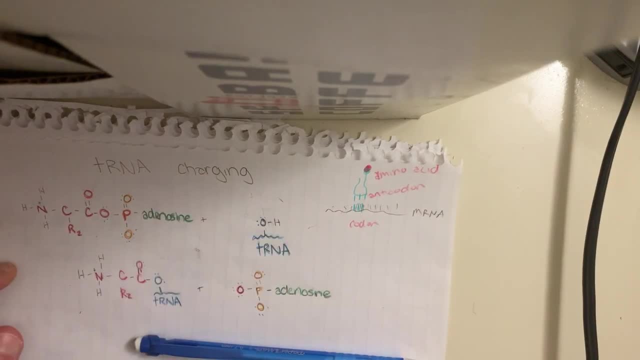 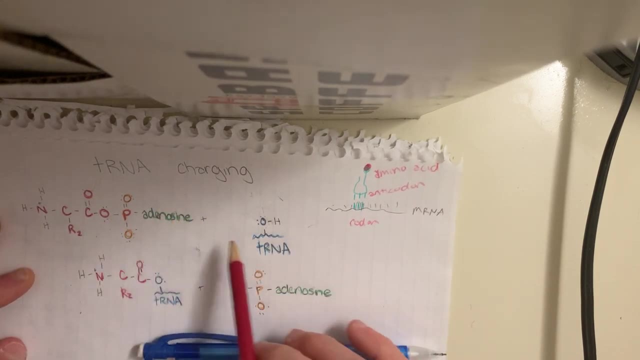 get the specificity. So different codons will give you different amino acids to be added And the tRNA is going to act as the intermediary between the two. So by charging the tRNA with the amino acid that we want to add, it's charging the specific tRNA that has the anti-codon that matches the 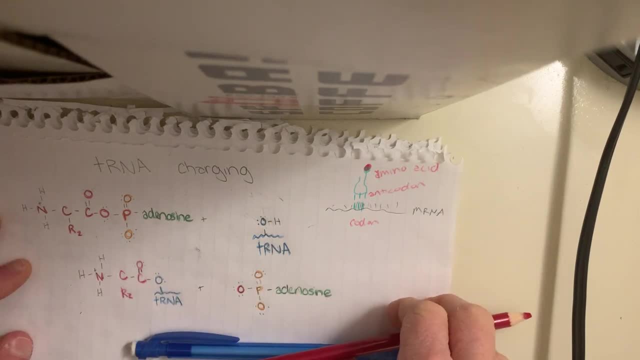 codon for that amino acid. So this is how we're going to get our specificity And so how's it going to work? So, like I mentioned, the tRNA really is. it really is RNA. So it's a form of transfer RNA. 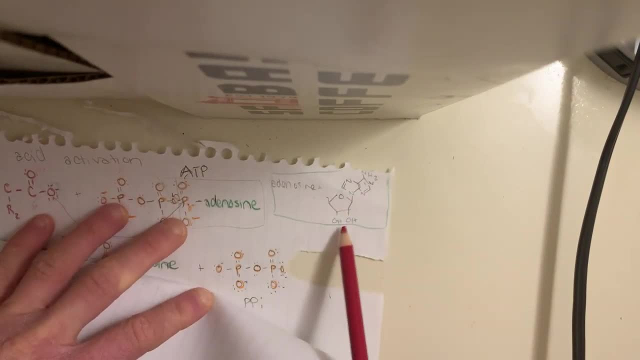 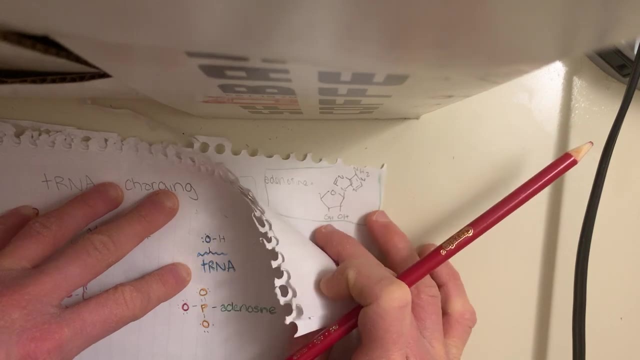 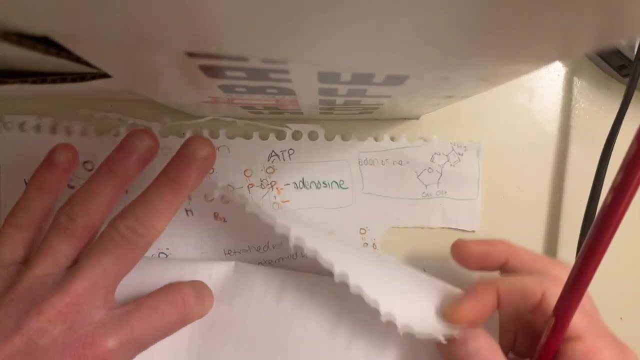 It has bases like this. They're not all adenosine, but so you have this ribose sugar and then one of these bases which can be A, C, U or G for RNA, And so it has just like this we saw with ATP. 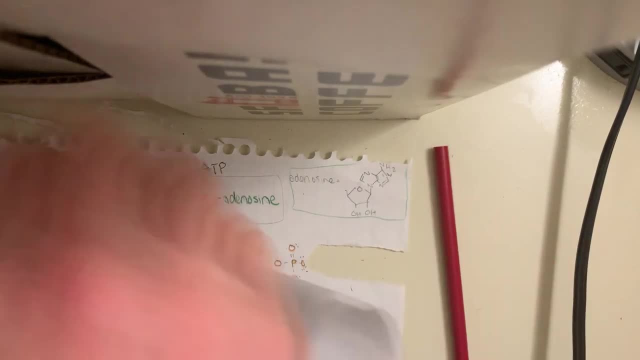 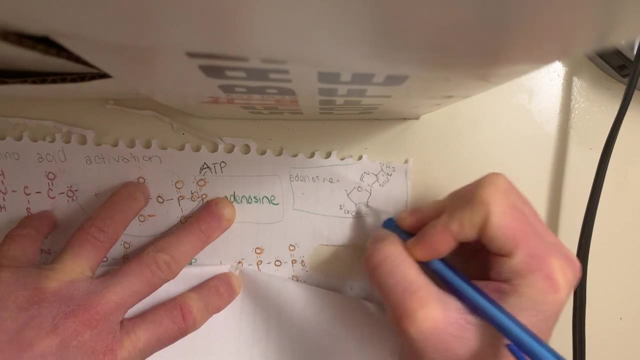 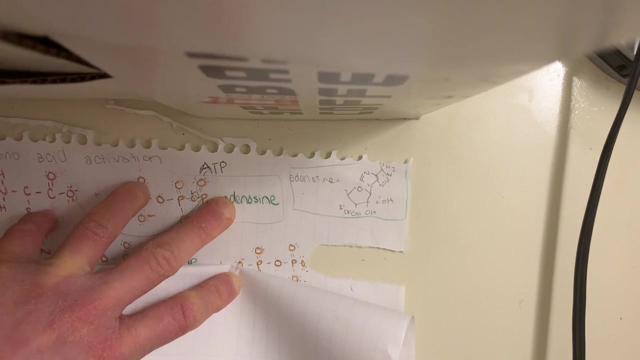 you have these two hydroxyl groups, And so this is going to be the. so this is the 3'OH and this is the 2'OH, And so this 2'OH is the one that ribose has, so RNA has, but deoxyribose, so DNA does not have. 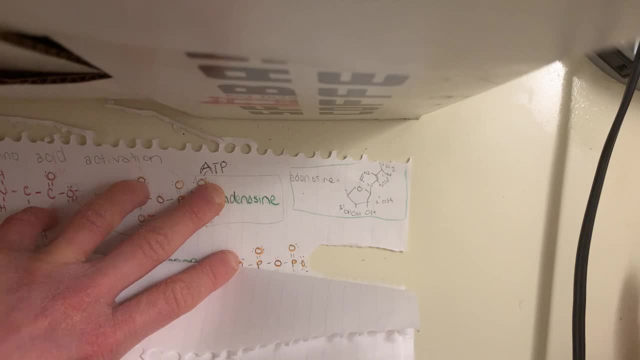 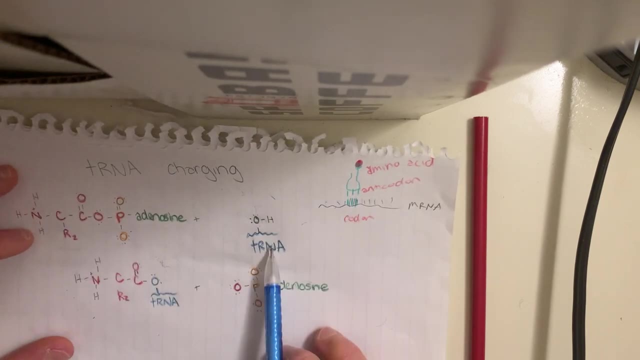 this OH here- And this is going to come into play later- as to why the ribosome, which is RNA, is able to catalyze this reaction, And so the tRNA. so we in that active site, we. so this is the. 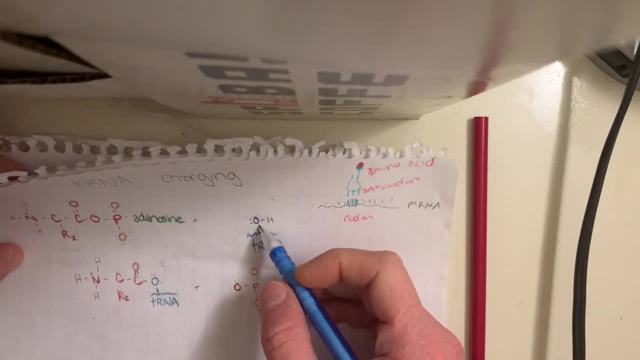 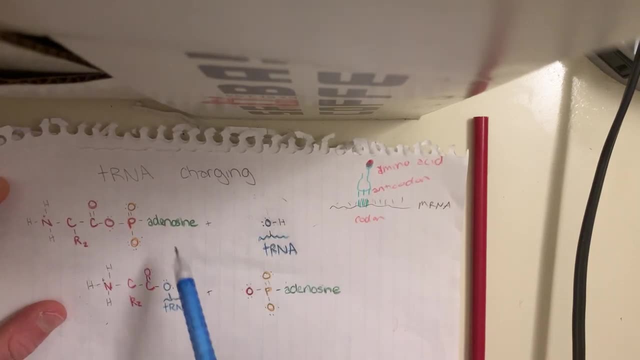 3'OH. So now it's kind of flipped upside down. But this is the 3'OH group, So this here It's the 3'OH group, So this here therapy, And it's going to now react with this. So we have 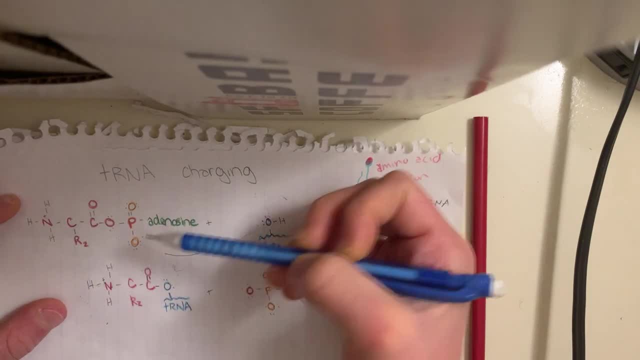 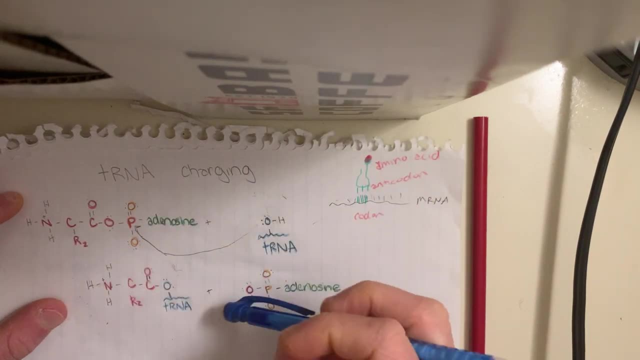 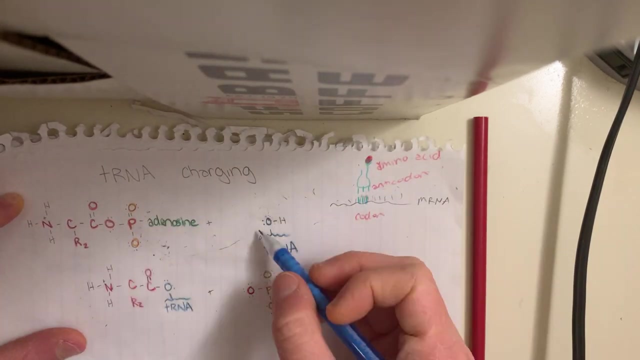 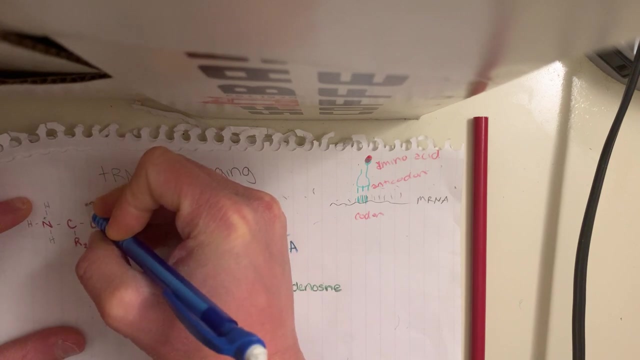 this oxygen with these lone pairs, You can get this nucleophilic attack onto this phosphate group. You can get this nucleophilic attack onto this carbon that you've activated. the oxygen is going to be pulling electron density, remember. so this is partly negative. 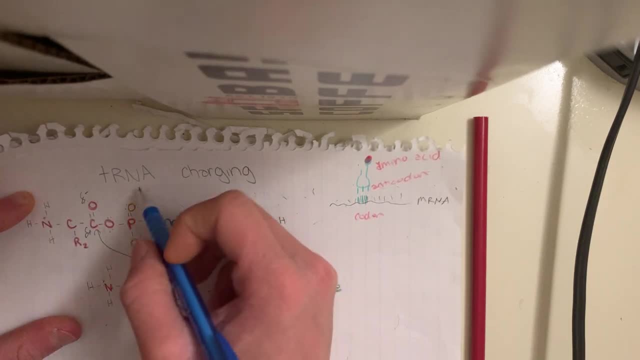 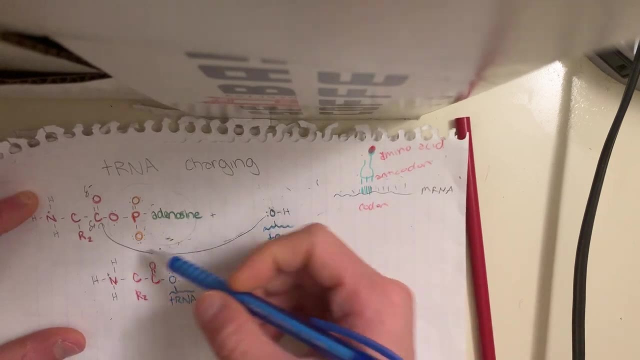 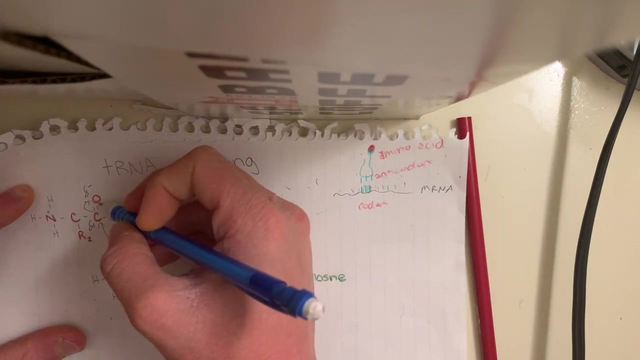 this is partly positive and this is a really good leaving group. so this oh is going to attack this carbon um and when that happens, the um, you get the electron flow, you get that intermediate like we got before. then that's going to um. so you get that um negative charge intermediate, which is then 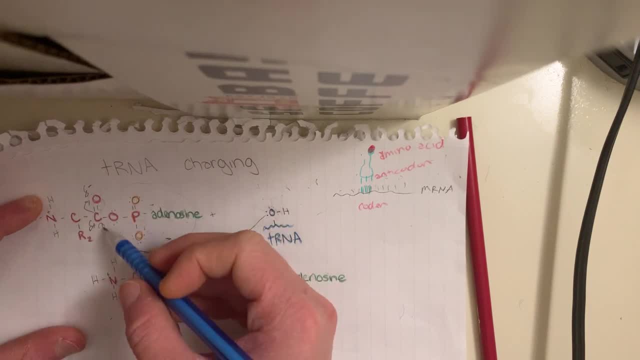 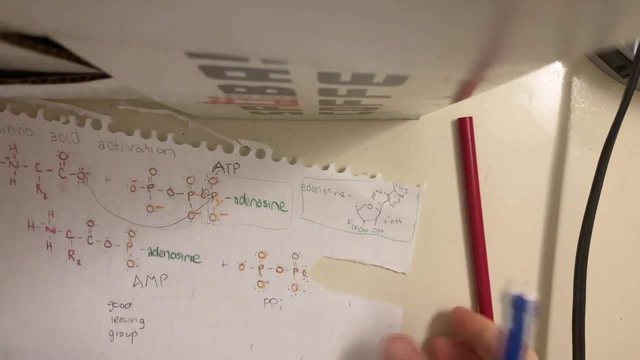 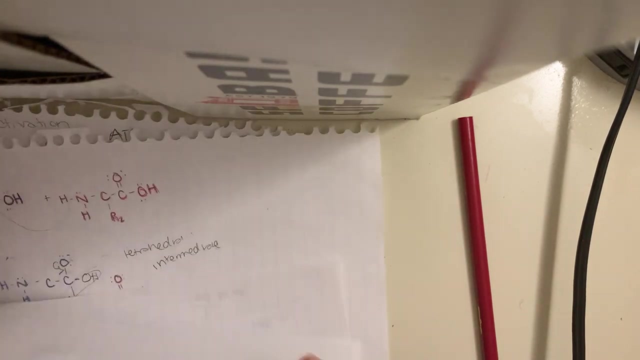 going to collapse back, so the octones will flow back down reforming this bond and you're going to get a leaving of this group. so now you've lost that oxygen. so going back to our very first thing about the, this reaction being a condensation or dehydration reaction, where you're actually 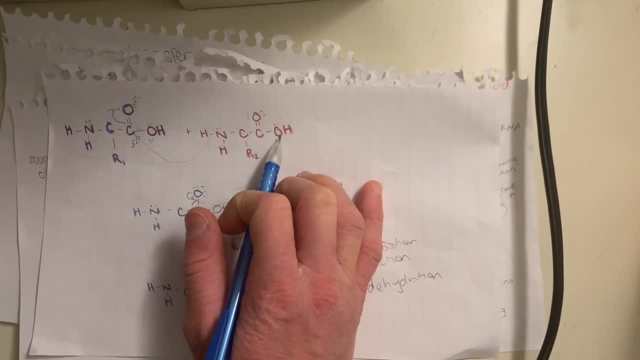 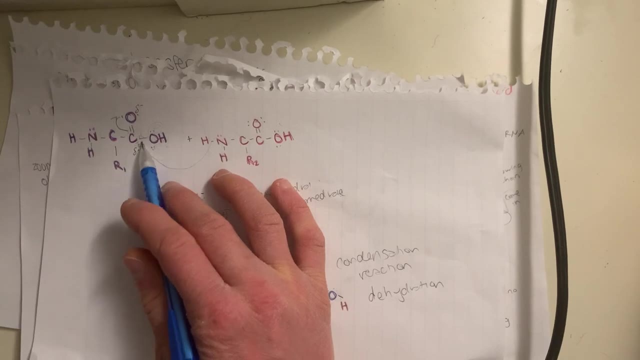 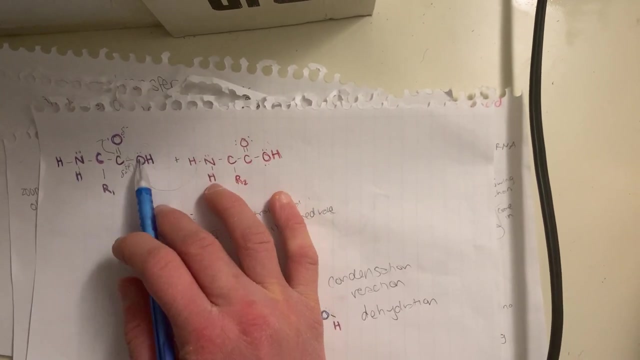 losing a water. so we're losing our water. see, we're losing that oxygen, this oxygen- this is the oxygen we're talking about. this guy is already like hooked up. this guy's already lost it's and it's attached to this growing chain. so it's happening in because these steps are separated. 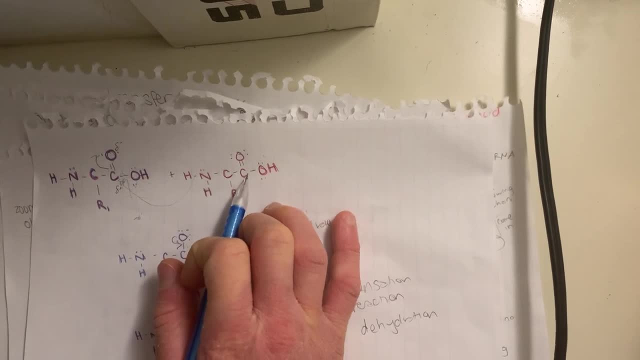 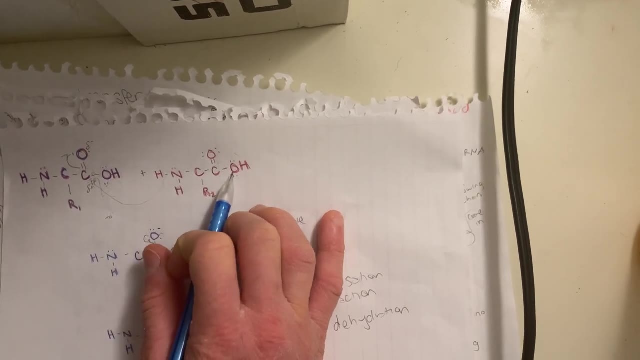 you're losing this group like way before you're actually going to um. add one onto this because, remember, this is the incoming and we just lost the oxygen from the incoming because we're hooking it up to a new oxygen with the transfer rna um. so it's kind of more confusing trying to figure out. 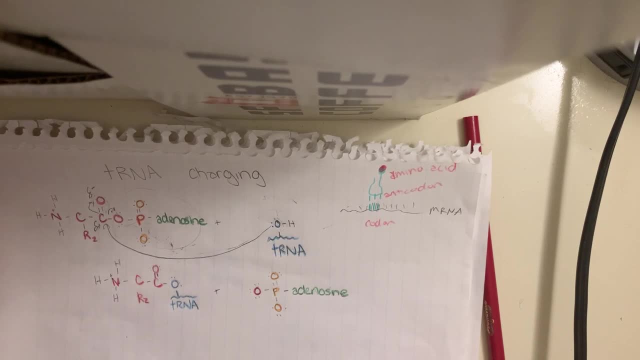 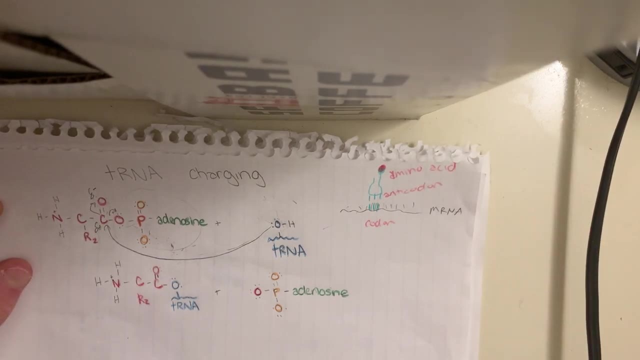 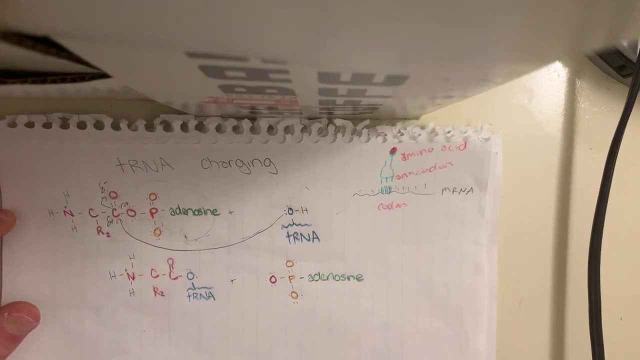 where exactly the hydrogens are coming from because, as i've talked about before, like hydrogens come and go, um, so, like h plus, they can leave, and come and leave it pretty readily, um, and depending on the ph of the solution and the pocket of the enzyme and all of these different things, um. so 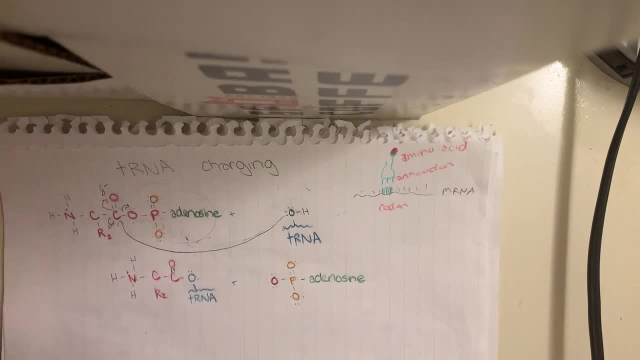 i'm not going to try to track the h's very much, which is why i haven't drawn them in color. um, but you do lose the equivalent of two ages depending on like what you start with. but um, because they can be in different protonation forms. but so just don't worry about what the h is really. 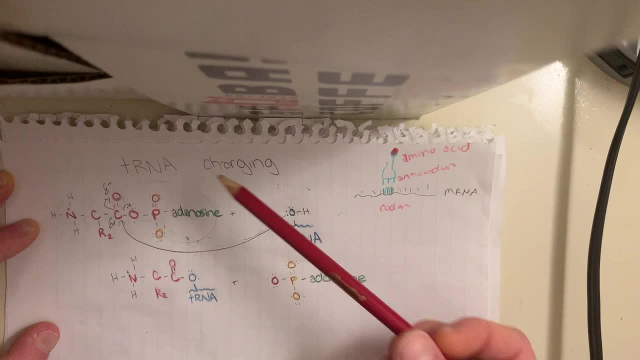 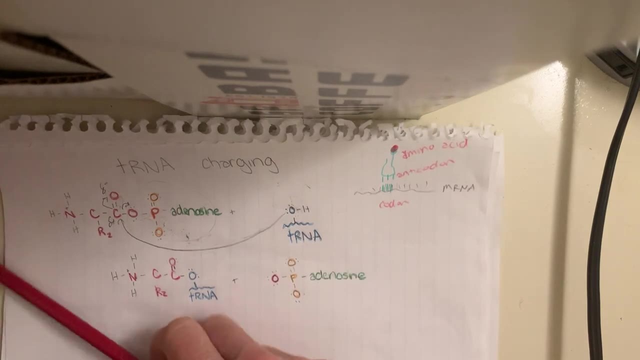 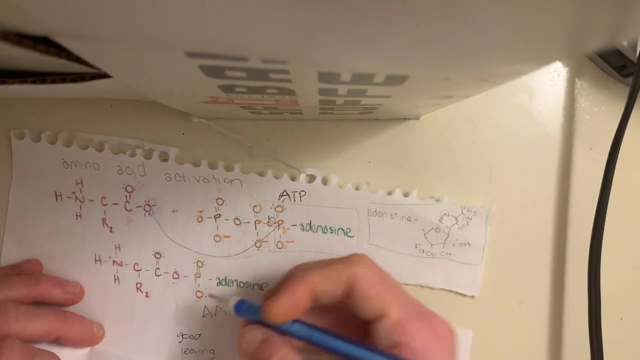 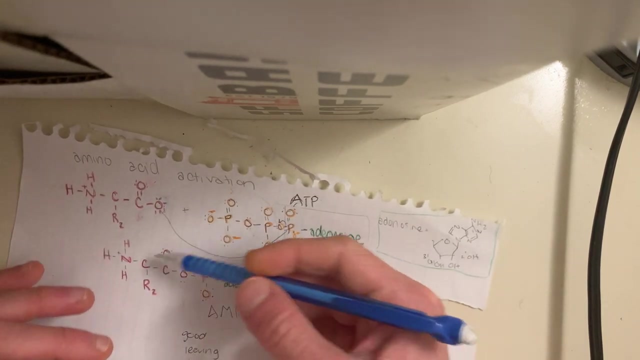 you're going to drive yourself crazy. um, so the ox, yeah, so now you're left with. so now you see, you've lost this oxygen. so this oxygen is now part of this amp, so this is amp. so we started with atp. we added this a. well, we kind of we added the um this amp onto here, and now the amp is free. 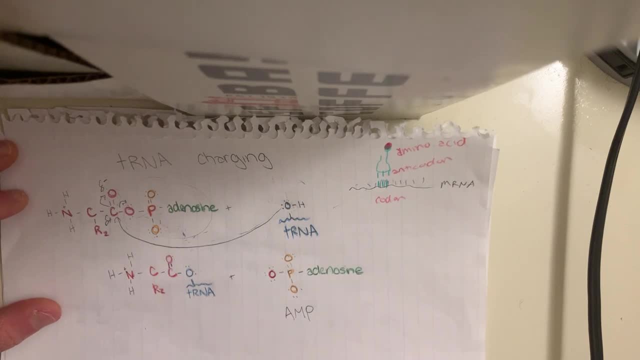 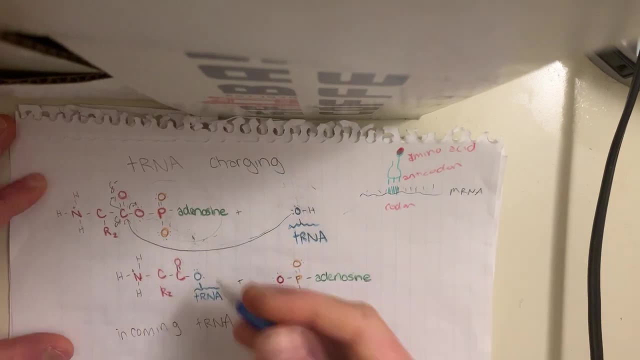 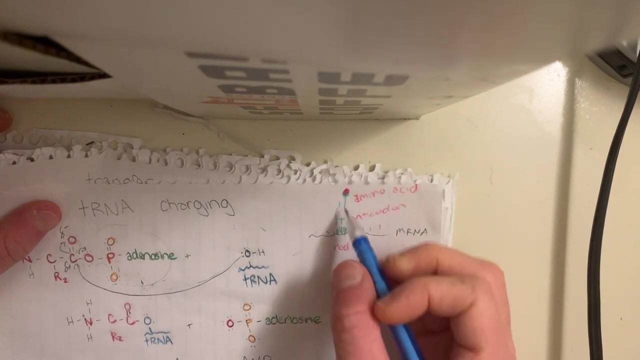 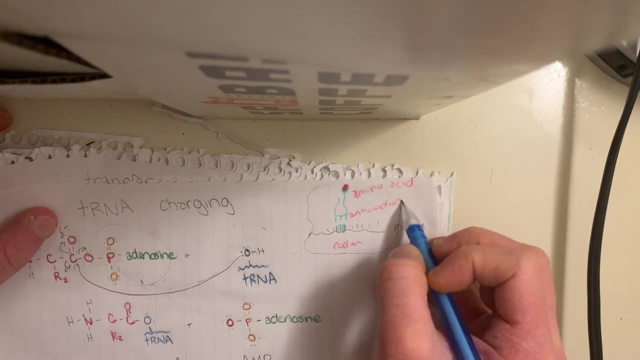 um, and we have this linked to this tRNA, and so this is going to be our incoming, incoming tRNA. and so now, when you have this um, so we have this codon, anticodon. this is all going to be take from now on. this is going to, so this is going to come and bind here and now everything's going to. 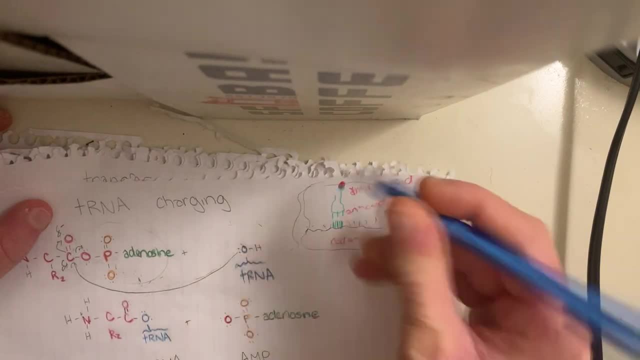 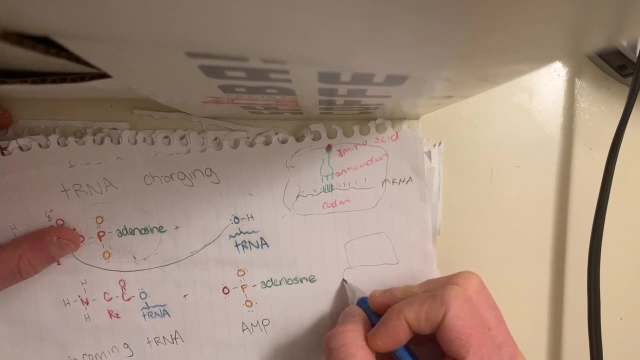 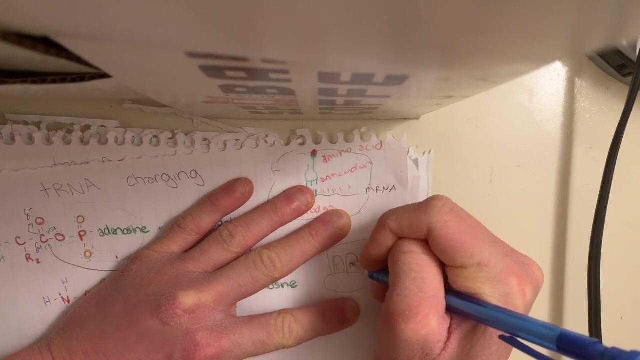 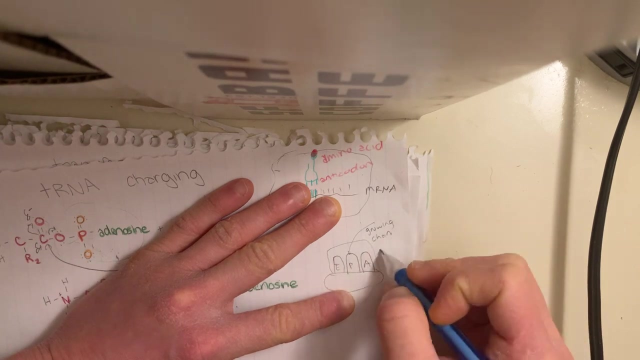 be taking place in a ribosome. so this big protein RNA complex and so this there's actually. the um has like several sites, so you have like these three sites you can think about. so you have the, the p- where's the growing peptide growing chain, the a- this is where it's going to come in. 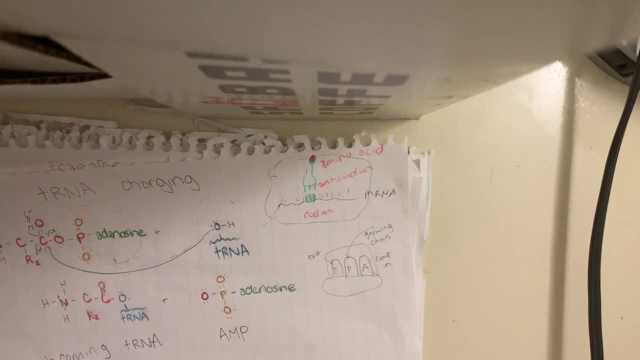 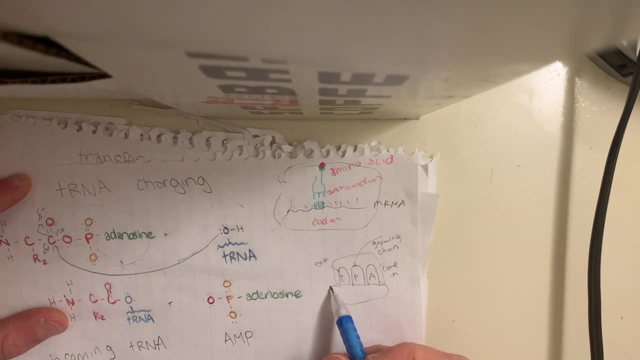 and the e. this is where it's going to exit, so our incoming one is going to be in this a site, the exiting one is going to be in the a site and the e site and the growing chain is going to be in this p and which where it's so p for like. 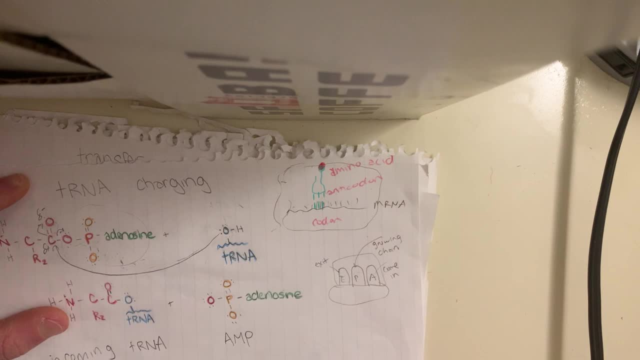 peptidyl transfer, um, because that's where the transfer is going to occur. and when I talk about transfer, so we have, we have the, we'll have the old tRNA and it's going to have this growing chain and then we have our incoming tRNA and it's only going to have this single. 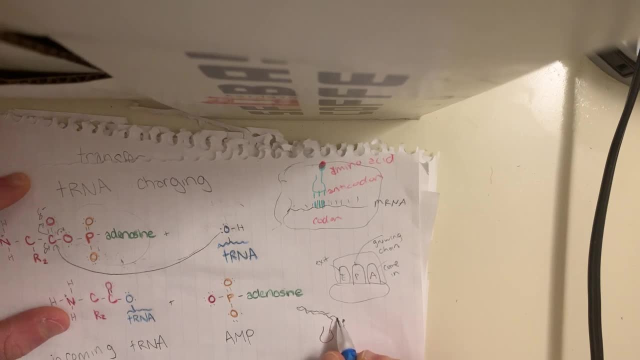 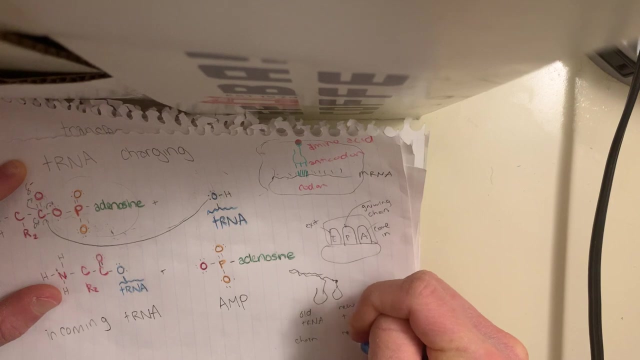 amino acid, and what's going to happen is this whole chain is going to get transferred onto this new tRNA. So this is going to be our old tRNA, which has the growing chain, and this is going to be our new tRNA, which has just the one amino acid. Okay, so this is the 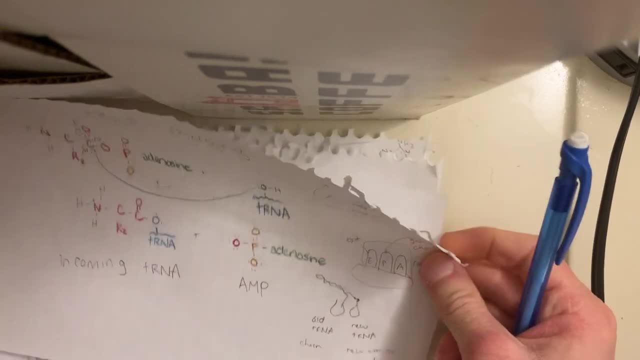 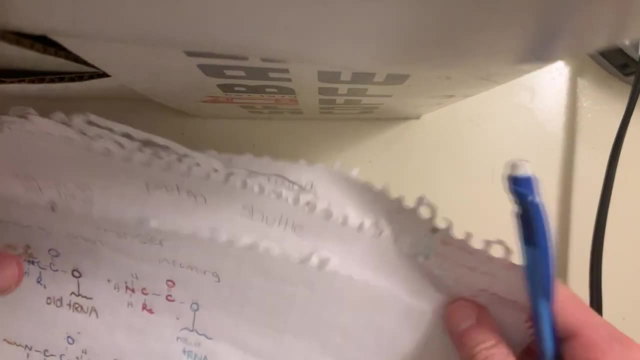 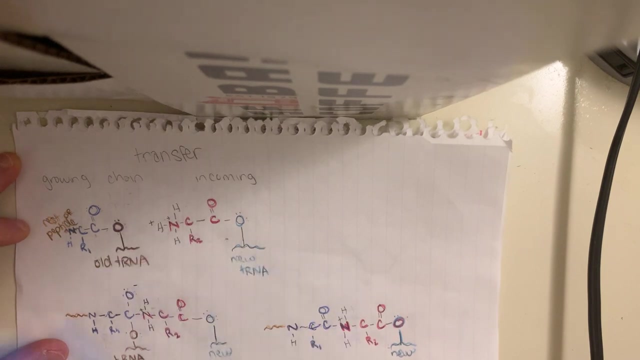 incoming. I'm just using old and new. So we're going to need to do that transfer and that's going to happen in the ribosome And so this transfer. okay, so we have the old tRNA. It's going to be attached, similarly to how we have the new one attached. So it's. 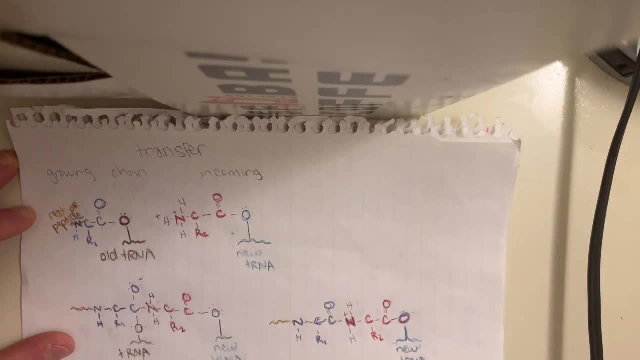 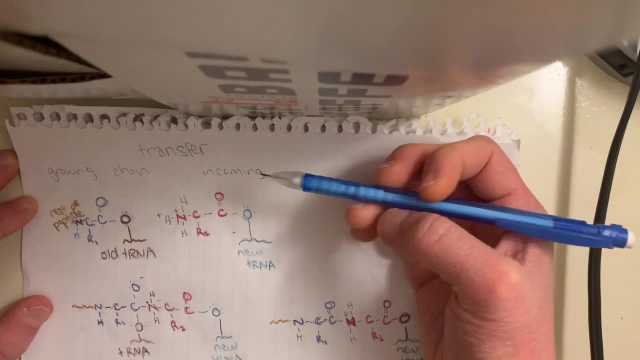 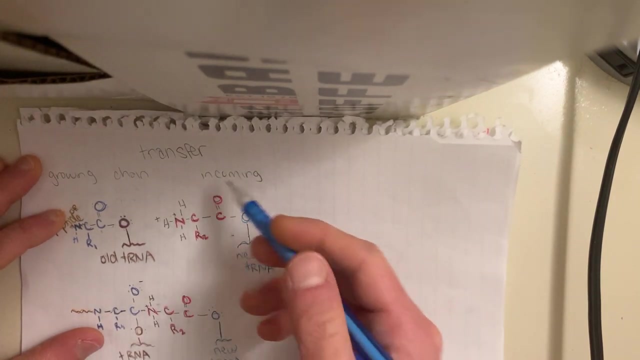 going to be attached to the tRNA site and what we're going to have is we're going to have this reaction where the it's going to be okay, so when it's in the enzyme, it's actually going to be when you have this reaction occurring. 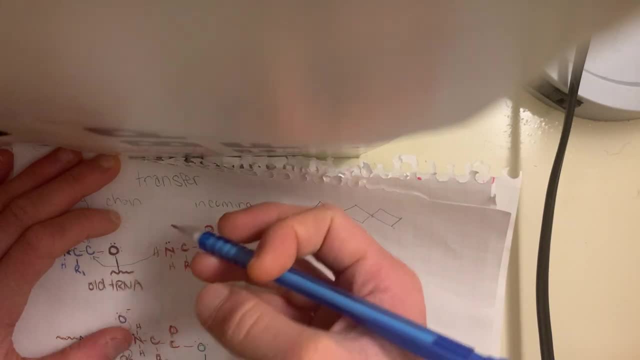 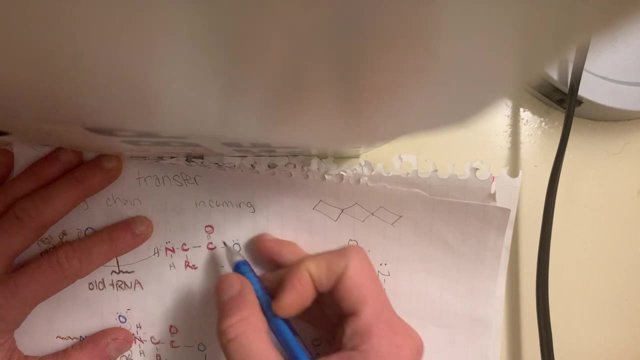 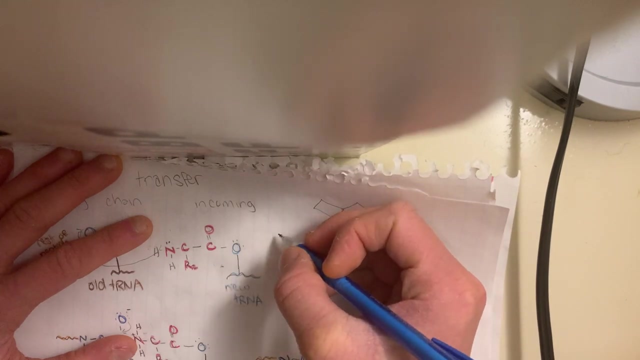 in like a pocket, like in the active site of the ribosome. So instead of the bulk water solution you have this pocket where you're actually excluding the water, So there's not as much water in there, And when you have less water, so NH3+ basically charged things. 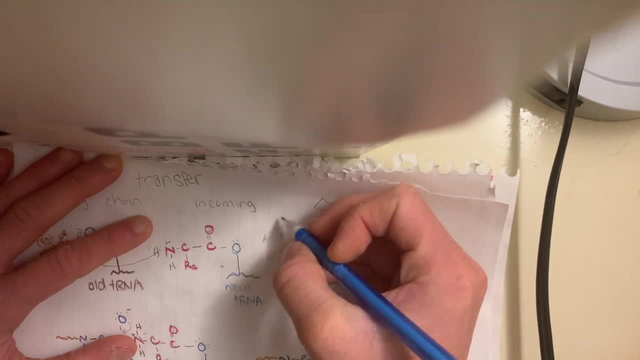 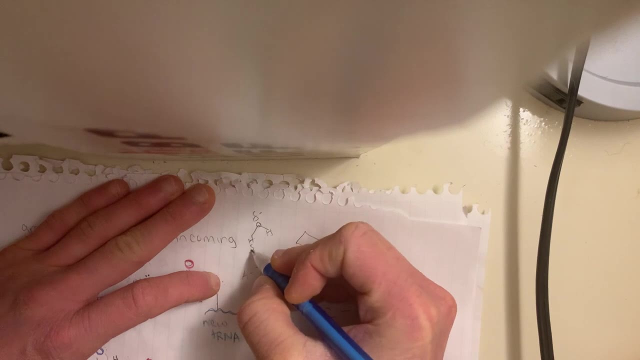 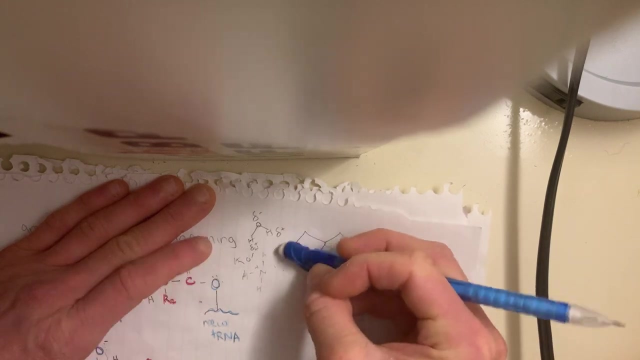 in general, water is pretty good. It's good at stabilizing them because water it has, it has the partial negative and partial positive parts, And so it can put its partial negative parts, it can orient itself so that it's kind of it's kind of stabilizing the positive charge of the nitrogen, And so this: 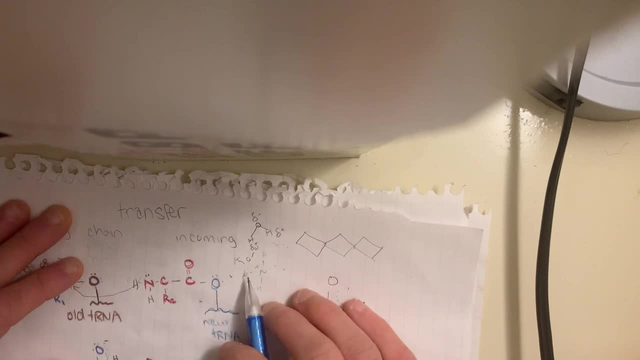 is going to make this more stable If you, and so that's less likely to deprotonate. however, if you remove the water now, this is more unstable and it's easier to deprotonate, And you also have this ester linkage is helping to like pull electron density and to lower 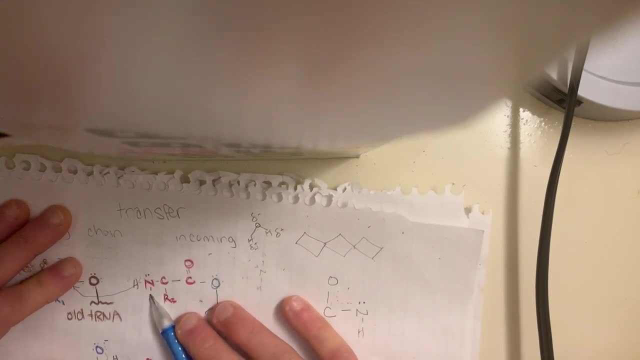 the, so you're basically lowering the effect of pKa. So it's going to deprotonate more easily when it's in the pocket of the active site versus when it's just Just free floating around. Remember, we need to have this in the deprotonated form, So 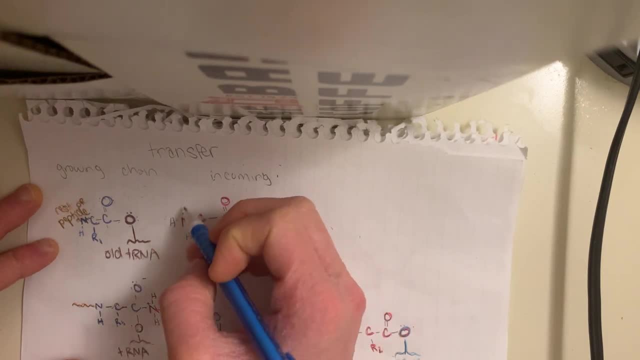 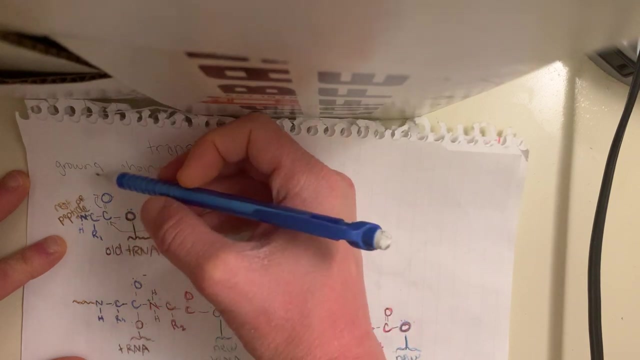 it has this lone pair of electrons that can act as a nucleophile and they're going to attack this carbonyl carbon, So similar to like to what we had before. So they're going to attack and this is going to generate this tetrahedral intermediate. 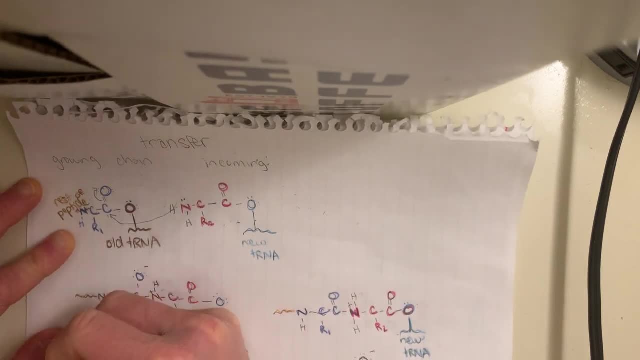 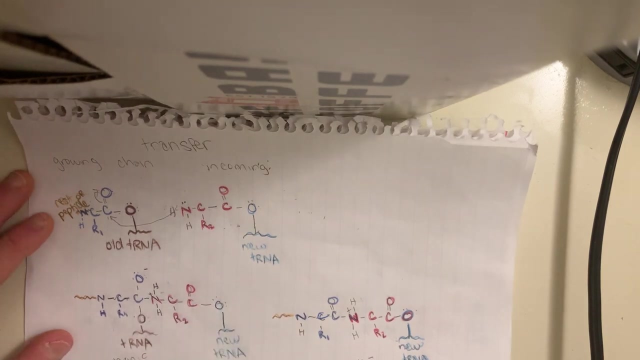 Like we saw before. So this is a little wider ionic tetrahedral intermediate And so tetrahedral referring to that this carbon is attached to four things. and sweater ionic, meaning that you have it's overall neutral, but you have a separation of two. 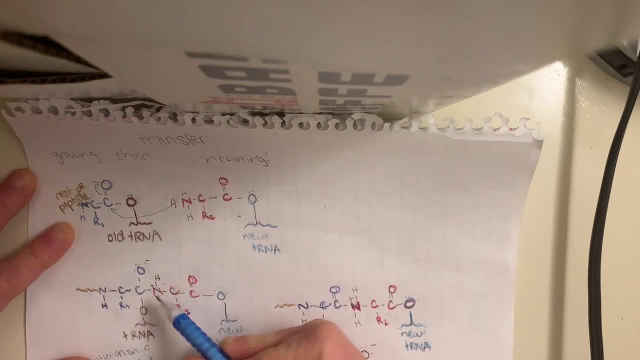 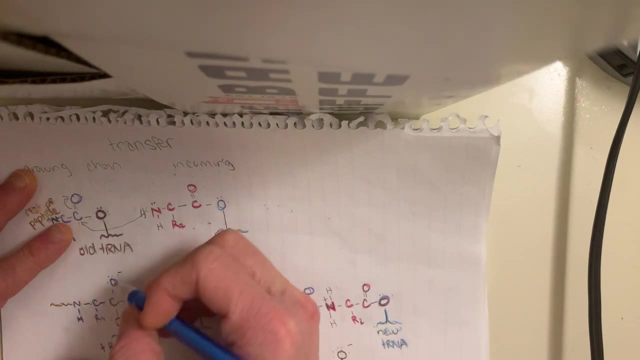 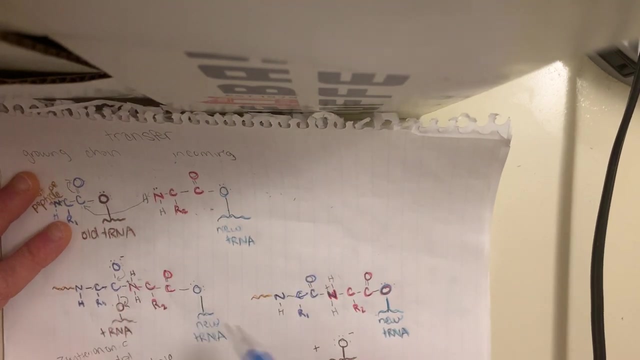 charges. So we have a negative charge on the oxygen and a positive charge on this nitrogen, And so this is a an unstable intermediate and it's going to collapse down. So these oxygens will come back to reform this double bond. The bonds from here will go to this oxygen, The electrons from that. 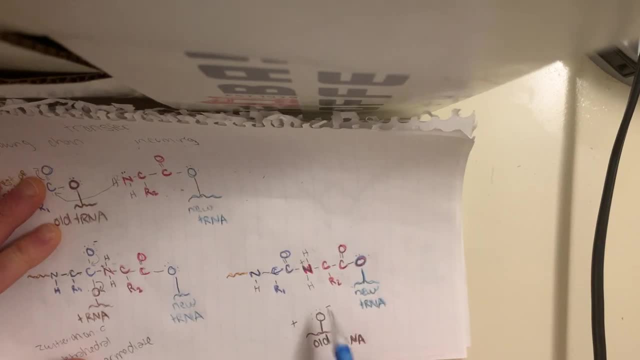 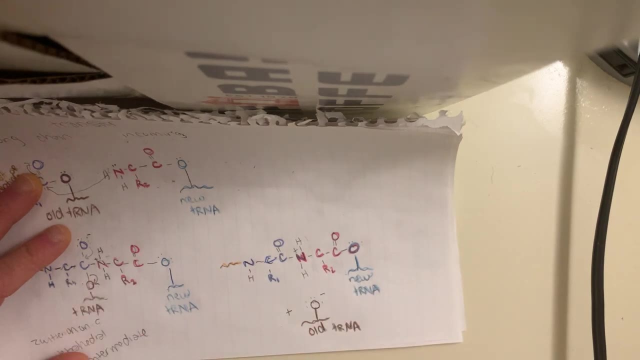 bond will go to the oxygen. And now your old tRNA: it's freed from the old tRNA and it's attached to the new tRNA And the old tRNA is going to have a negative charge because you move those electrons onto here And you can see that. but you still have this. you still have this charge. 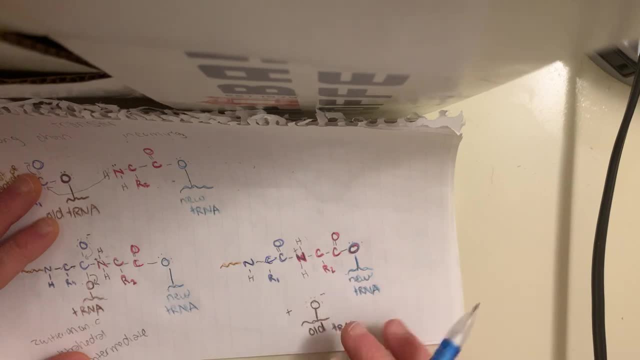 on the nitrogen. So the nitrogen is attached to four things And so it doesn't have like five, like so when it has a lone pair it would have one, two, three, four, five electrons attached or assigned to it. And it likes having five because it has five protons. But in this state 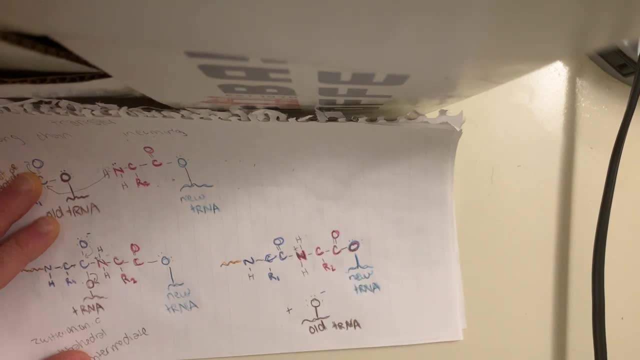 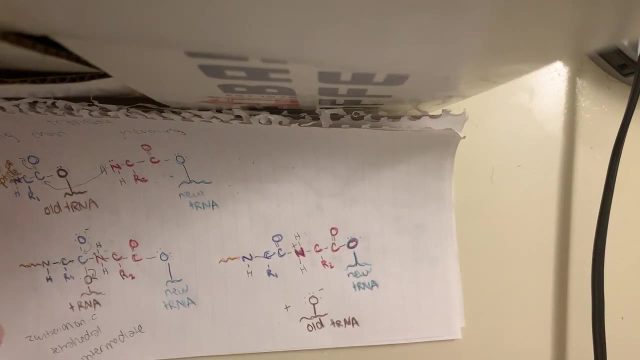 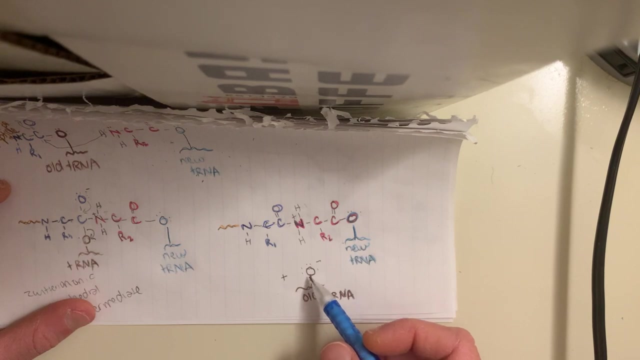 it has four, And so that's one less, Then five, And so it has a positive charge because it has, yeah, because it has those five protons, So it has this positive charge And this is not going to be found in our peptide. 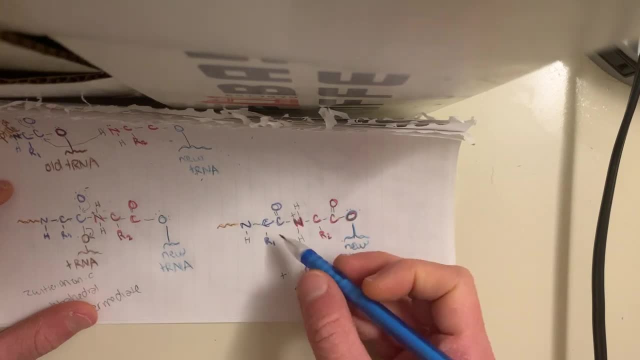 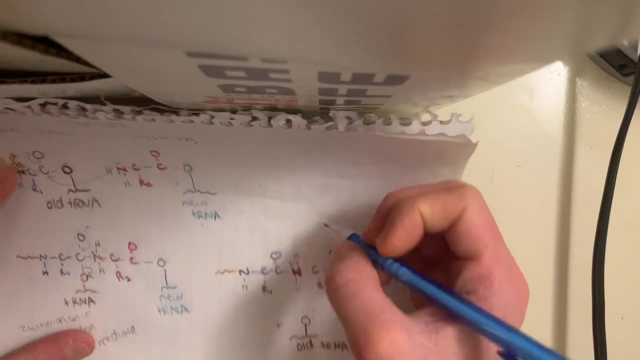 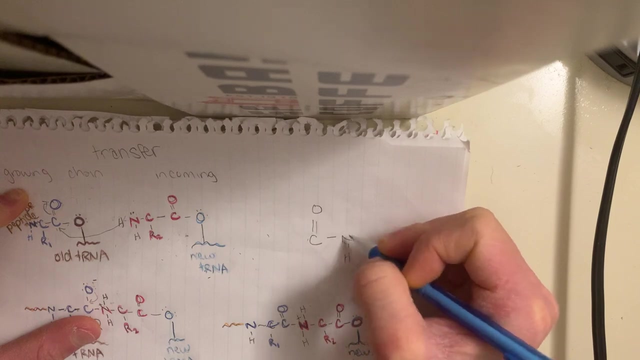 And it's important that it's not going to be found in our peptide bonds, because in a peptide bond you actually have resonance stabilization. So between so this lone pair, when you have a lone pair, when you have, When you have this, you have this lone pair. you're going to actually have resonance stabilization. 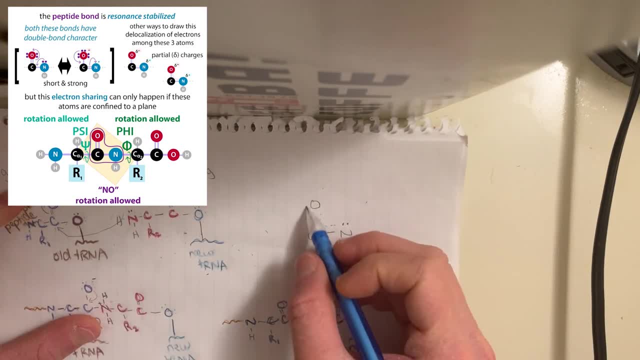 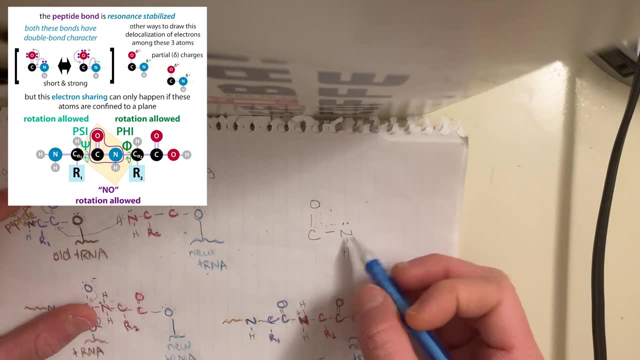 between these. So you have partial double bonded character of both of these, with the, with the sharing of these electrons, And that's going to provide stability And it's going to provide a, it's going to provide for the backbone, It's going to make the backbone like sturdier and 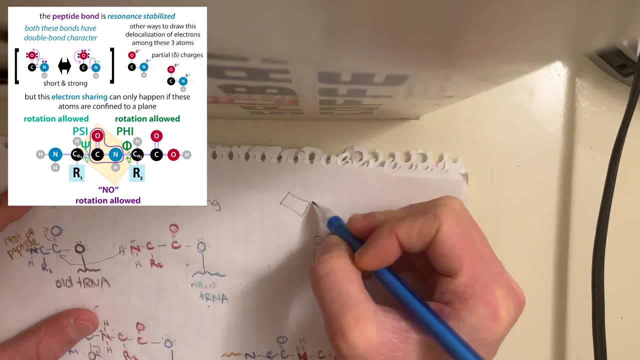 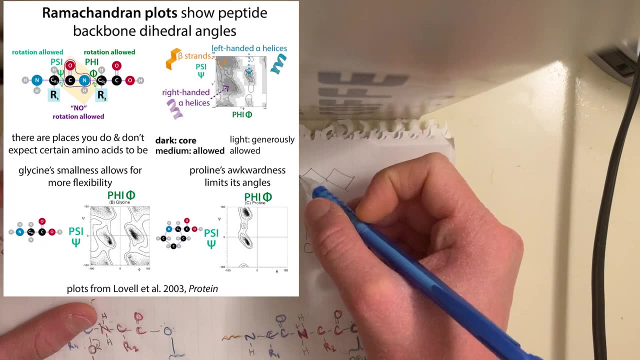 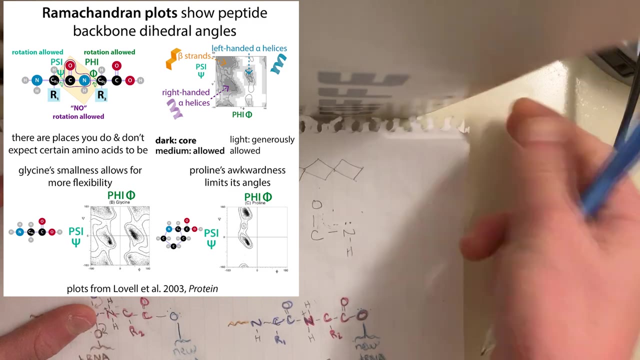 have, it's going to limit its rotation. So you're actually going to end up kind of with a plane of planes And depending on how bulky the side group is for the amino acids, you, you can get various degrees of rotation around those planes And this is going to allow proteins to form like 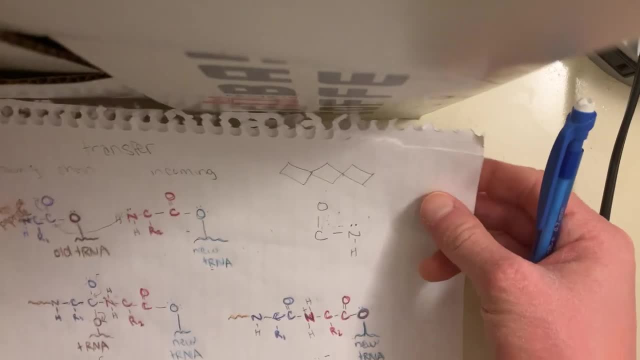 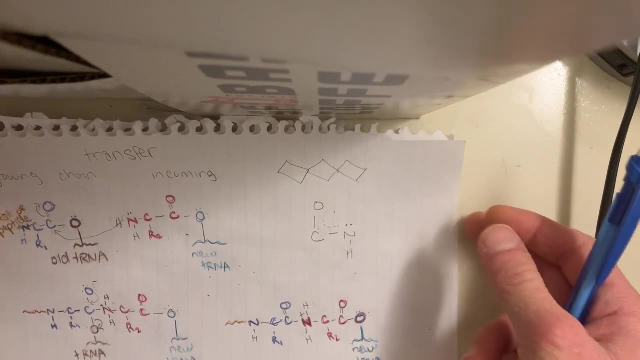 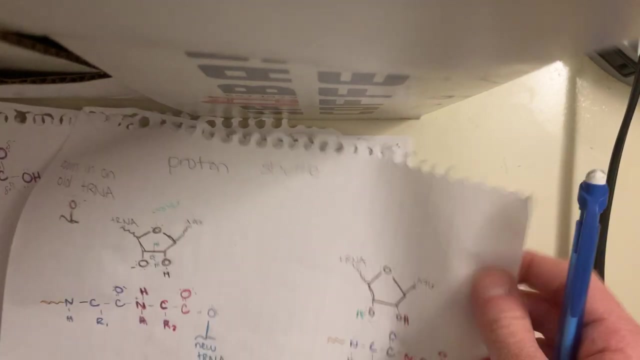 characteristic secondary motifs like helixes and sheets. But to do that we need to deprotonate this hydrogen, this nitrogen, And this actually happens, split to happen through this, like proton shuttle mechanism. And so if we zoom in on the old tRNA, so now 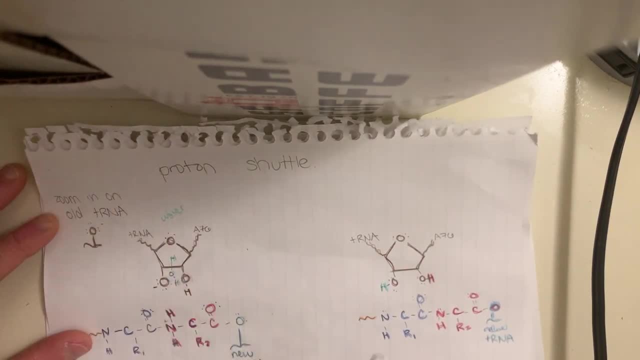 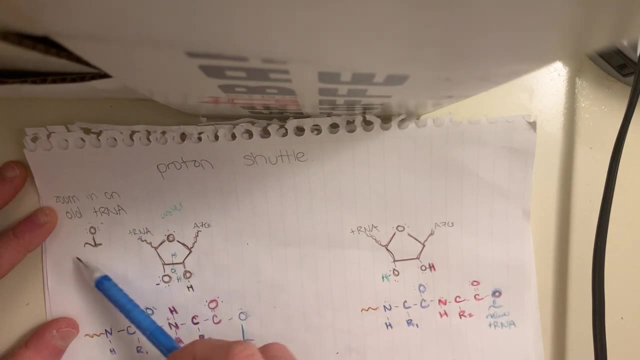 this. now I've kind of flipped this over, Sorry, but the so, if you look at this, like so, this was our three prime OH. So this is that, now this, and so our two prime OH is here. Yeah, so I just sorry, I was basing it off of a figure. 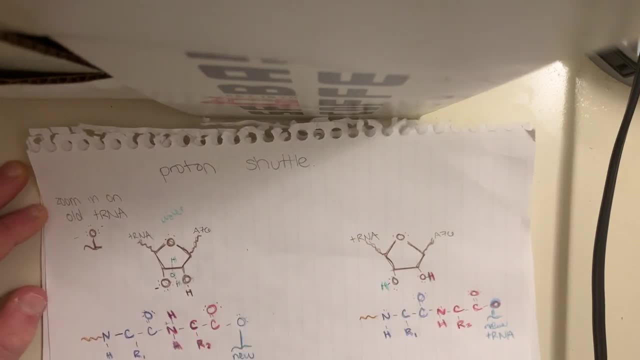 So if you look at this like: so, this was our three prime OH, So this is that, now this, and so our two prime OH is here. Yeah, so I just saw it was basing it off of a figure, of an N. 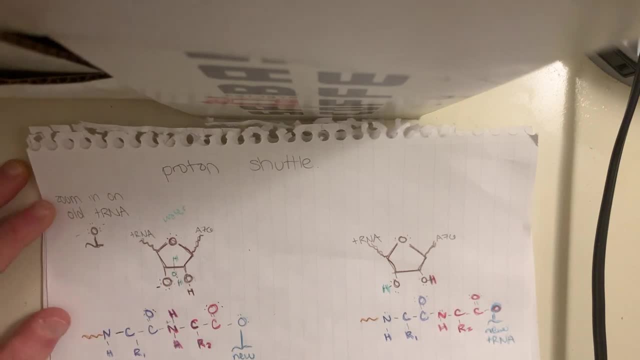 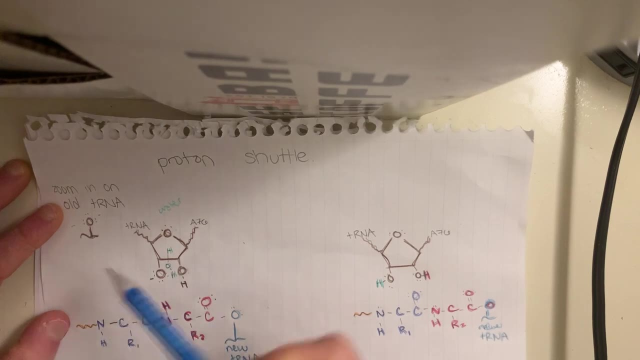 figure, but that figure was drawn differently than other figures and so hopefully I got everything okay But this. so this is your 3'OH and you would think that this would just like pull off that proton, because negative, positive, this one would take that H, but 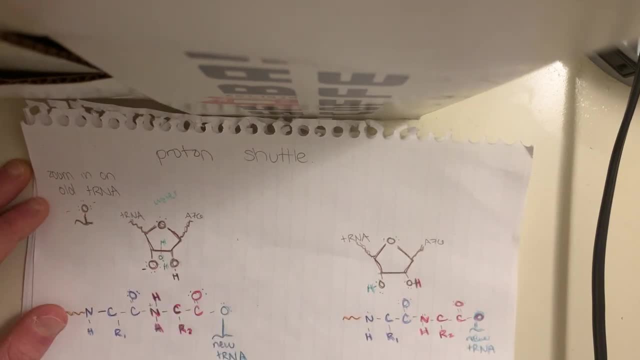 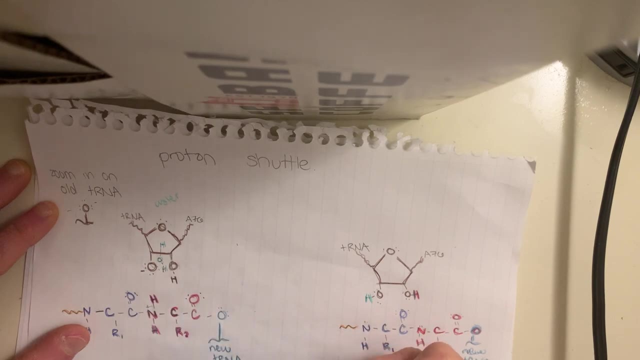 it turns out it's more complicated, because in like structures of this you can see that it's only that this is too far away to pull that off, whereas the 2'OH is near enough to pull it off. but the 2'OH is already protonated, And so it turns out they think that the OH 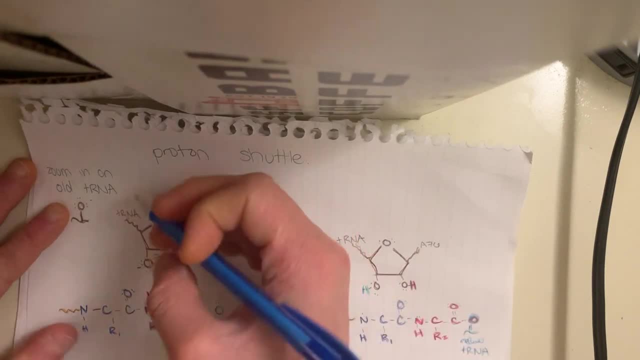 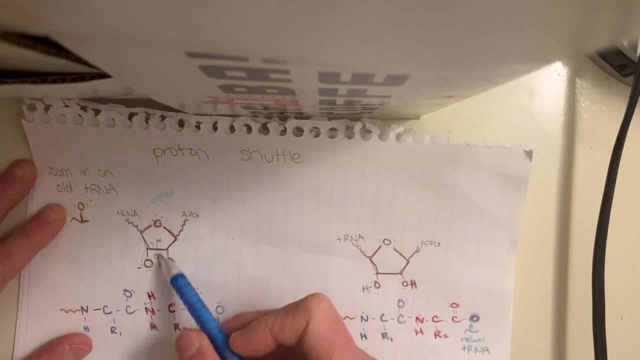 so that this oxygen is actually going to take from this coordinated water. so this is. there's a water molecule here too. so if you're looking at that on paper, you might get kind of confused, because there's a water molecule sticking out like this and you're like what the heck? 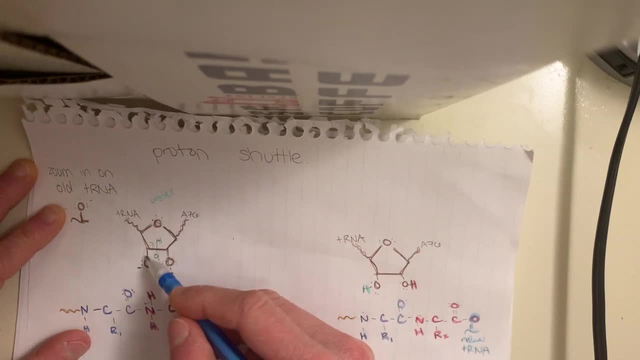 is that, Because it's all drawn the same color There, that's a water, And so this can pull a proton off of that water and then that gives you OH- OH- can then take a proton from here, so this one becomes O- then that can pull a proton from. 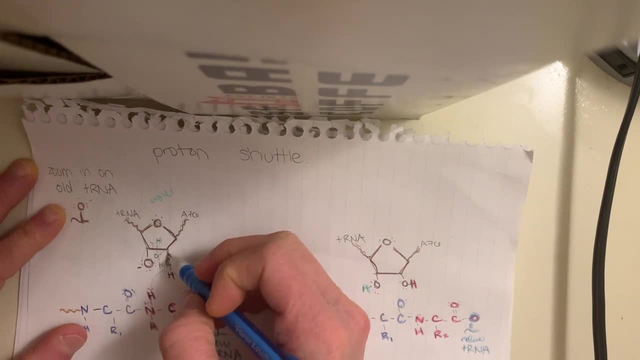 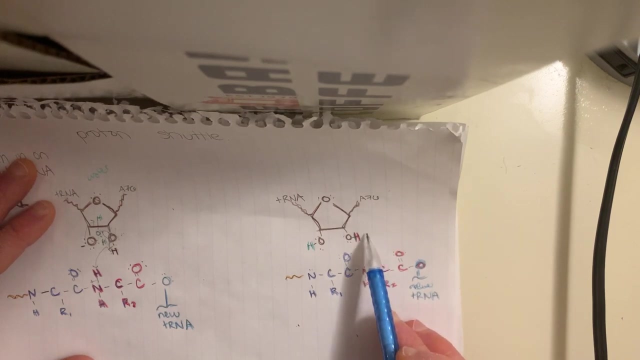 here. so you have this very complicated way to get this back to its protonation step. But so it's this. it's called a proton shuttle, Um, And so now you're left with. you have your tRNA, you have that regenerated, you have. 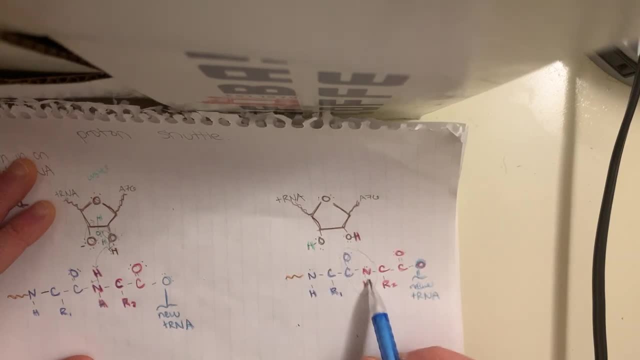 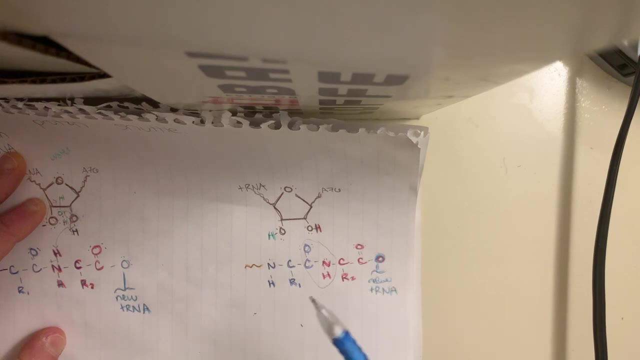 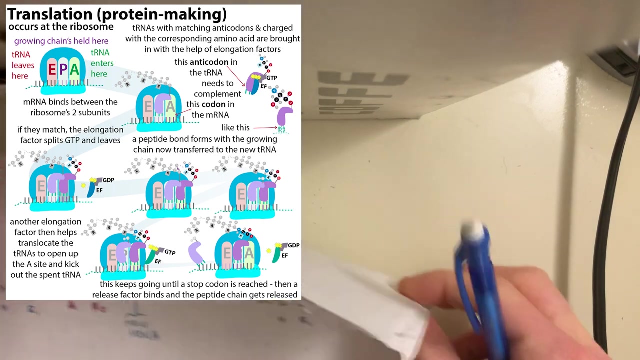 your peptide bond with the ability to have that resonant stabilization. and now everything is attached to this: new tRNA And then um. with the help of like elongation factors and things this is going to get shift. this all shifts into the um P-site, so where the growing chain is on your amino acid um. 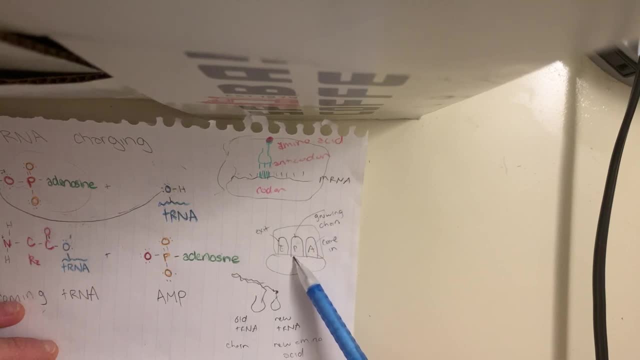 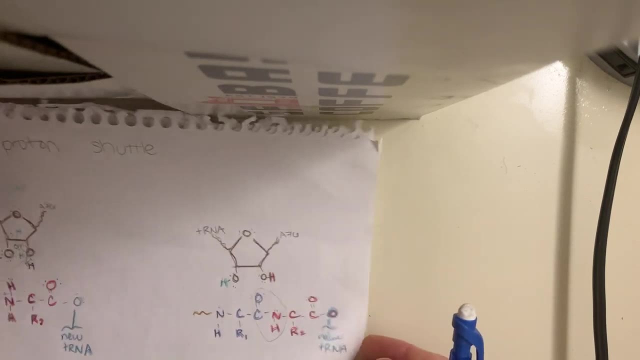 of your ribosome. So this is going to shift and be in this um, the P-site, the growing chain, and then a new one's going to come back in. So overall, we have the same um, we have the same end product, as we would see if we just 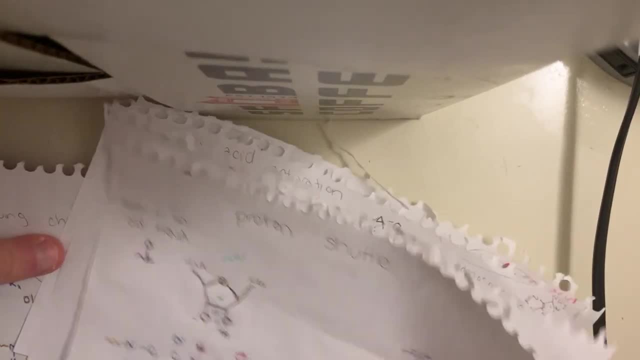 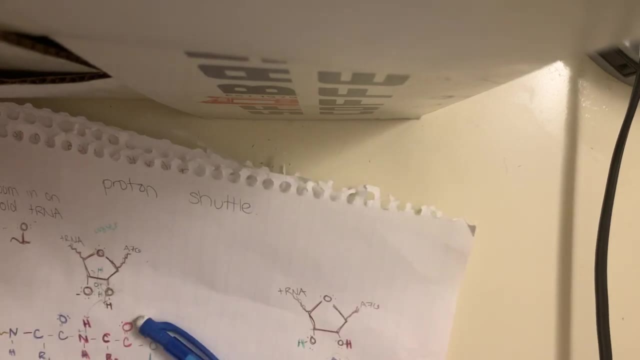 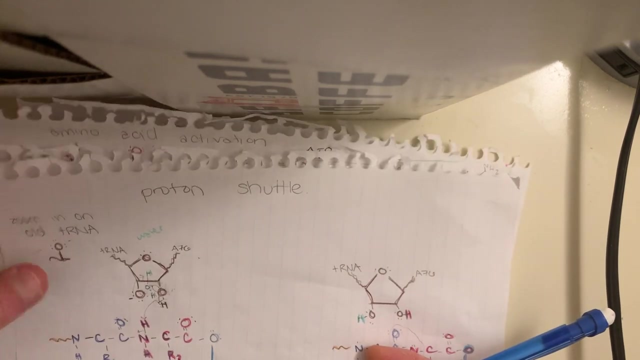 looked at, um the basic overview of the reaction, except that we are doing this, um in a sort of convoluted way, taking these different steps Um in order to first so activate the amino acid, so give it the energy it needs make. 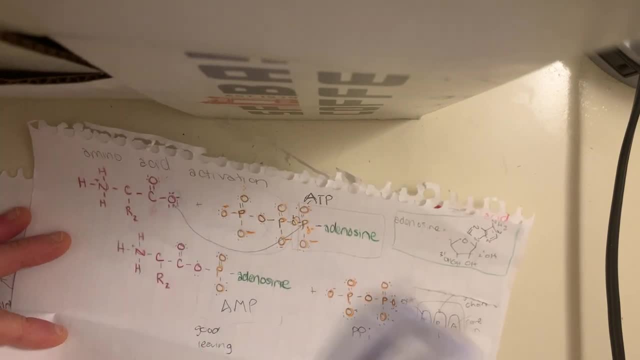 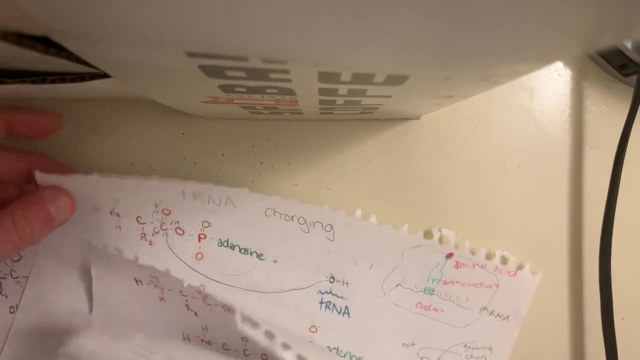 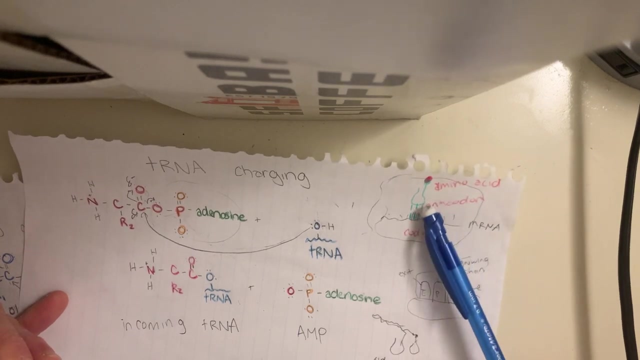 that carboxyl um, make that carbon more reactive um and by adding this better leaving group, then we're going to charge the tRNA. so we're going to this is going to give us the specificity that we need um going from so that the right amino acid is added that corresponds. 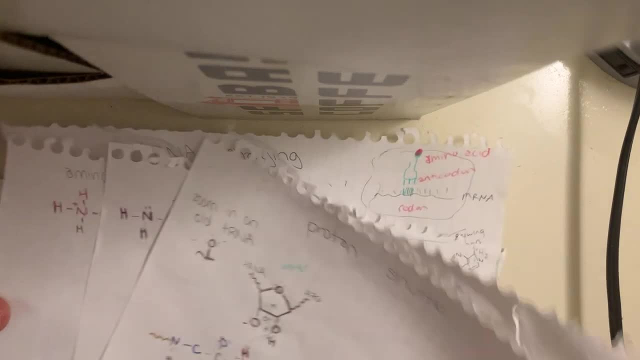 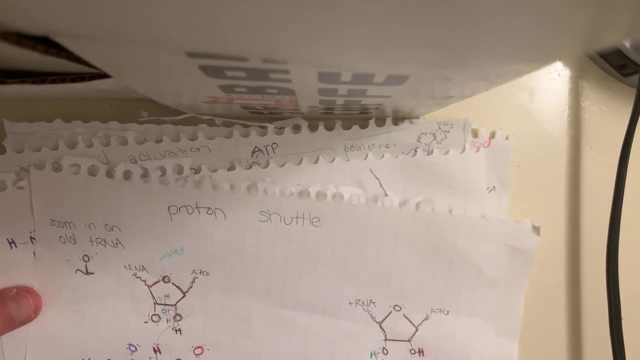 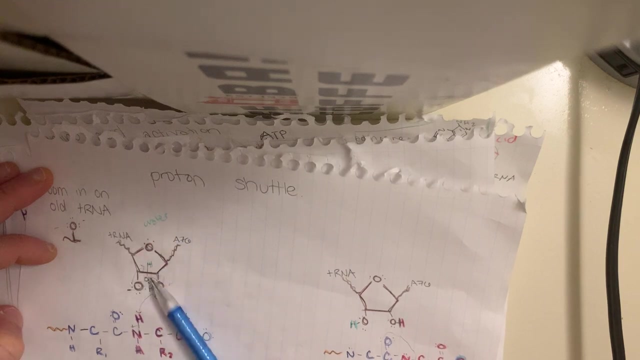 to the mRNA, Um, And then, Finally, we're going to, with the help of the ribosome and um, we're going to facilitate this reaction and make it happen. Another cool thing. So this is showing you like the tRNA that's helping, um, the old tRNA, how it's helping. 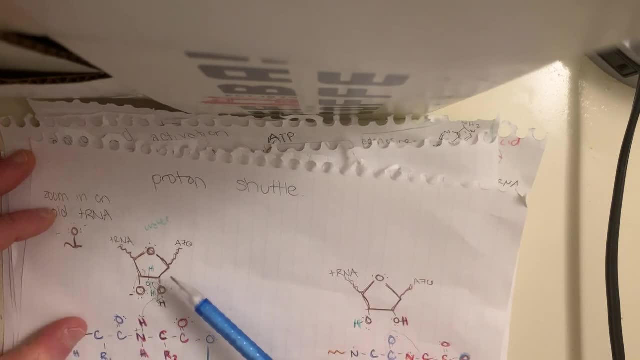 with this proton shuttle is um. so it turns out that if you have, because this OH, this two prime OH, is participating in this shuttle, this reaction is not going to work if you have the DNA um there, So if you have a deoxyribose there,